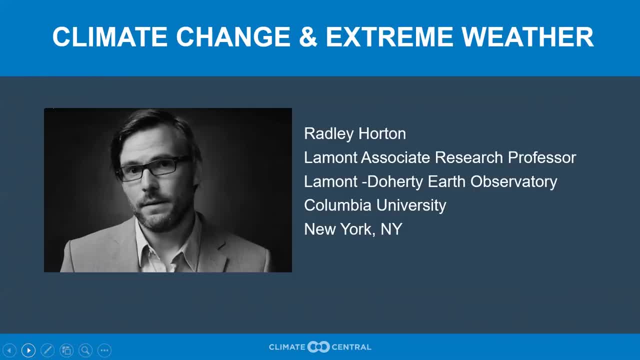 including the Climate Scylene Awards Task Force in support of the 2018 National Climate Assessment. As a brief aside, we want to encourage questions for Radley at the end of the presentation, So please use the chat function on your Zoom platform at the bottom right. 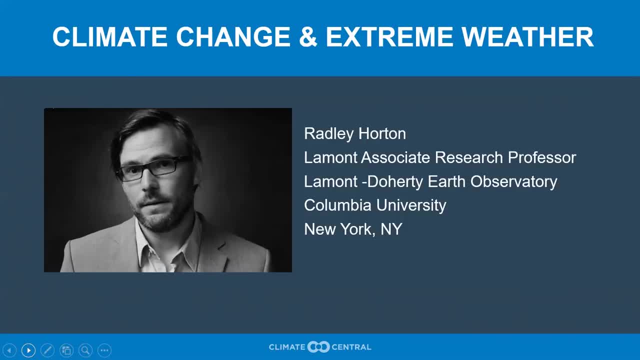 Type in your questions and we will get in as many as we can during our 60-minute time limit today. With that, Bradley, you still with us. sir Bradley, can you hear me? I'm sure you're not muted on accident. 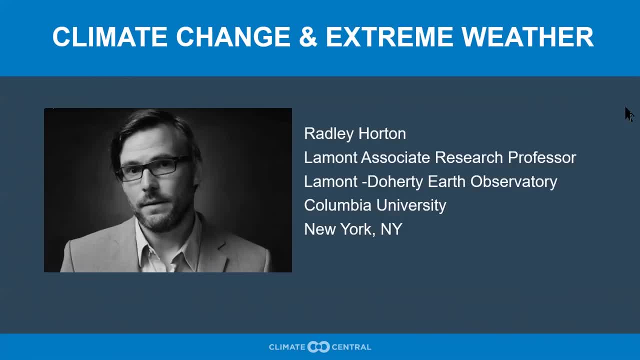 These things happen. There you go, sir. I apologize for that. Can you hear me now, Bradley? Yes, Can you hear me? I hear you just fine. Sometimes you know you have 40 different buttons to push. These things happen. 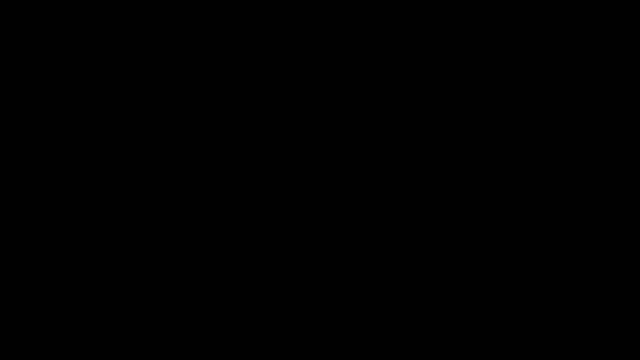 So I'm going to stop sharing. This gives you the opportunity to share your screen, So go ahead and do so, sir, if you are ready. Okay, See if that will work. Share screen. You're not seeing my screen yet, are you? 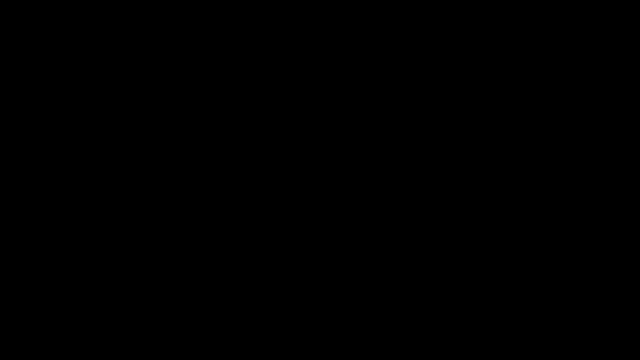 Not just yet. Okay, So I'm getting a prompt that says Host Disabled Attendee Screen Sharing. Well, that's odd. I'll make you the host. Let's see what happens. Okay, So let's see here. Great. 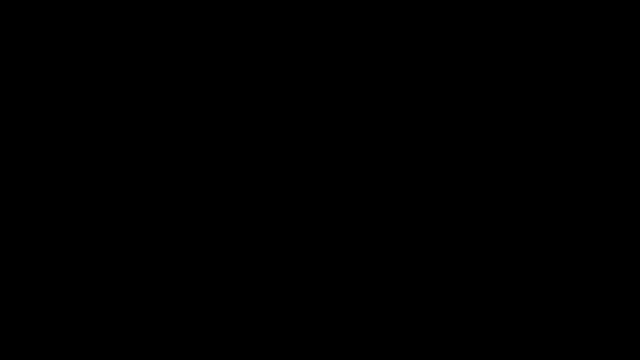 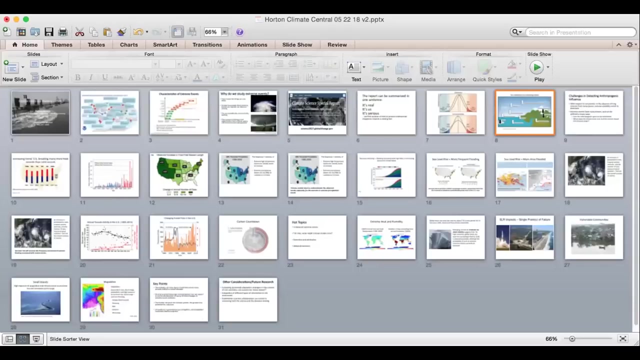 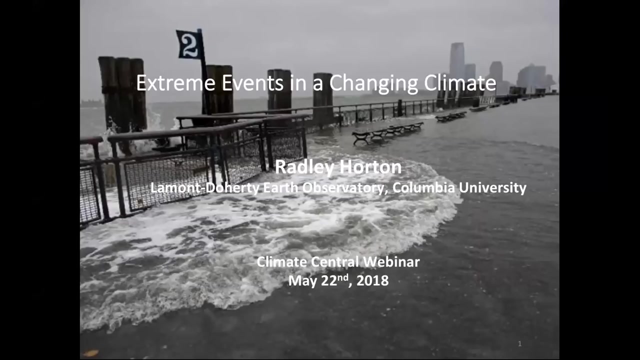 I think this is now going to work. You can find my presentation in the midst here. Yeah, there, we are All right. We've got it over here, sir, Okay Okay. Thank you everybody for patience during that. 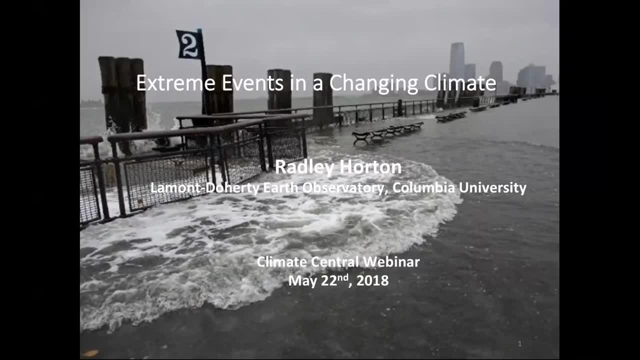 Really happy to have the chance to speak with you today. I am going to focus largely on extreme weather events, a key interest of mine at Lamont-Dowry. I think a lot about the key processes, what goes into. you know what are the ingredients? 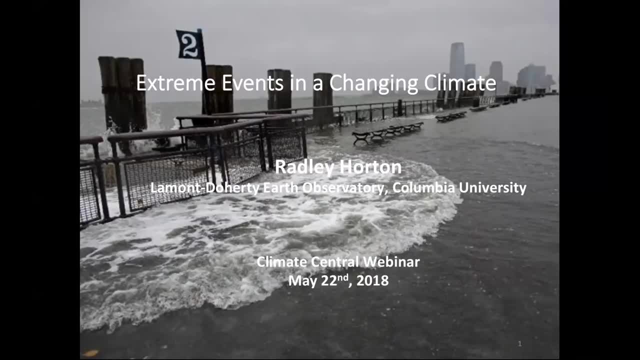 that formulate these extreme events that have such big impacts on our society, and how might they change as we increase greenhouse gas concentrations in the atmosphere through our activities? During most of the talk today, I'm really going to focus on what we've observed to date. 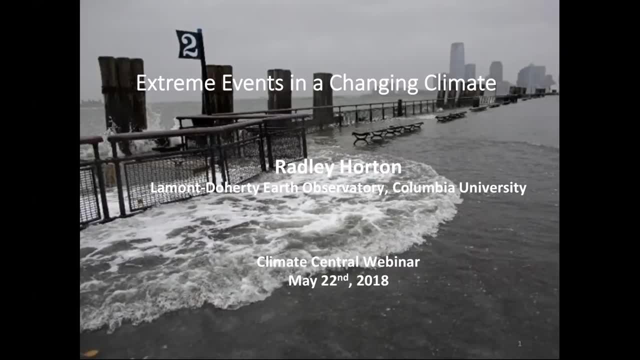 sort of historical dimension to extreme weather events. So there'll be, you know, a fair amount on some of the time series- largely for the US- of extreme weather events, But we'll also have some time to talk a little bit about things like: what does the future? 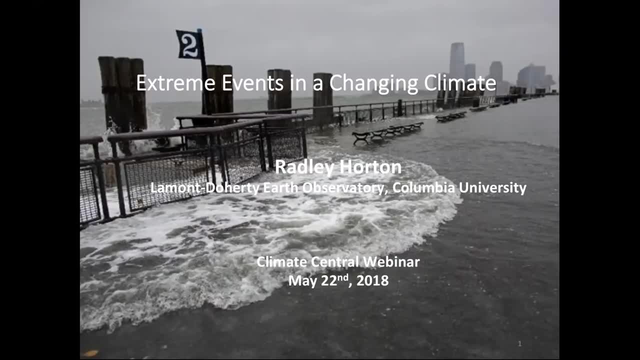 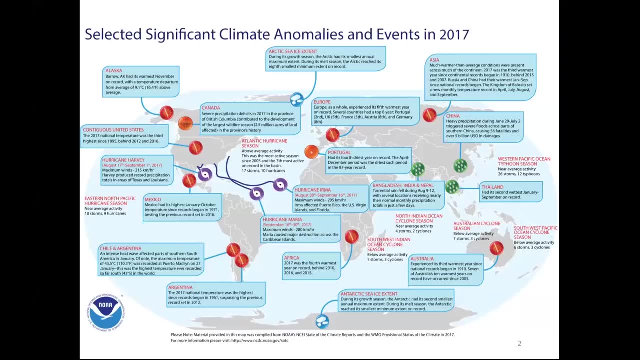 look like. What are some of the limitations of what we can tell with climate models And some of the impacts and how we may adapt. Okay, does everyone see? did the slides just advance? We look good from here. yes, sir. 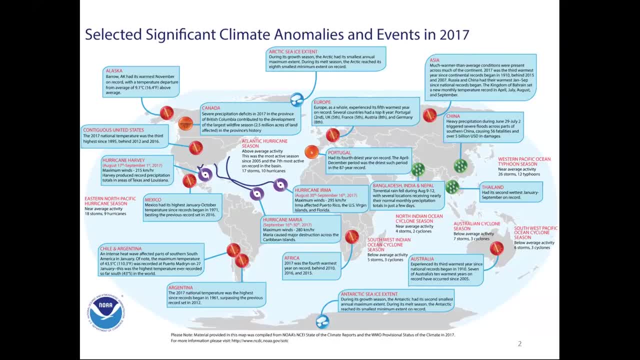 Okay, great. So you know, as in any year, if we look at the global scale, we see a diverse set and diverse types of extreme weather events. You know some things that certainly jump out at us and are fresh in so many of your memories, I know. 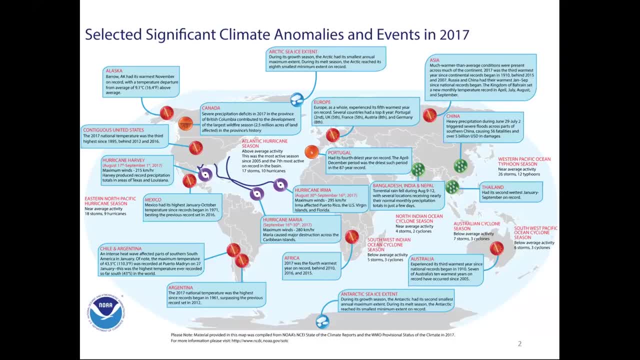 The hurricane season over the Atlantic last year, reminders here of Harvey, Irma and Maria, which by some estimates, if I remember right, may have caused on the order of 300 billion in damages, not to mention the hugely significant loss of life. 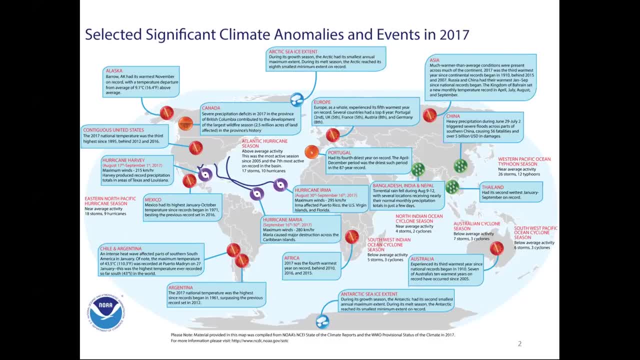 So that's the context, you know, as we think about, about extreme weather events. they're diverse in their type, They impact the entire globe and, by many indications, their costs are going up, presumably partly due to, you know, changes in human vulnerability, human population. but we're 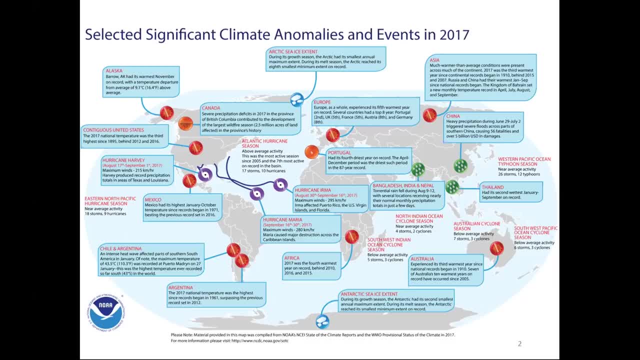 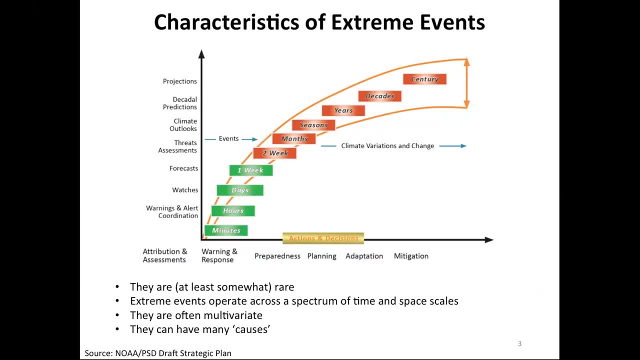 also going to try to unpack climate signals as well within these extreme events. So what are some of the characteristics of extreme weather events? Well, they really are diverse, as you can see here, in terms of time duration and spatial scale, Depending on what type of events we're talking about. this could be a microburst, you know. 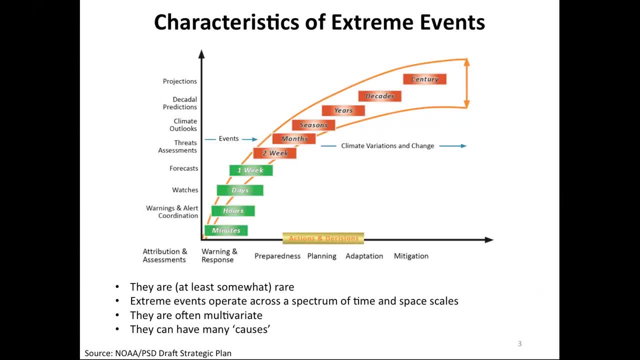 a really high-resolution rainstorm, the kind of thing that develops and persists, maybe over a few minutes, at very fine spatial scales. We could also, of course, think about extreme events as multi-year phenomena. in some case, you know, really severe droughts such as California has experienced, and events that may have spatial scales. 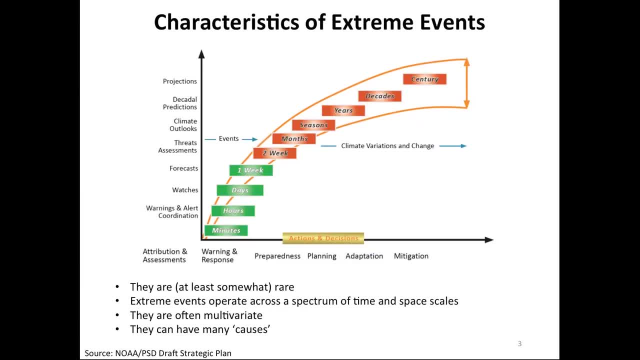 you know the size of the US or half the US, so they're very diverse. Pretty much any definition that you'd have of an extreme event, you know, would start from the assumption that it's at least somewhat rare. 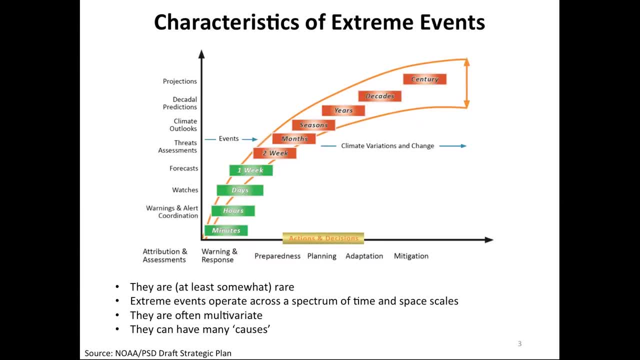 You know, is it something that happens once every several years in a given place? or is it, you know, days above 90 degrees Fahrenheit, which for some places, might happen as often as you know, 30 or more days per year? 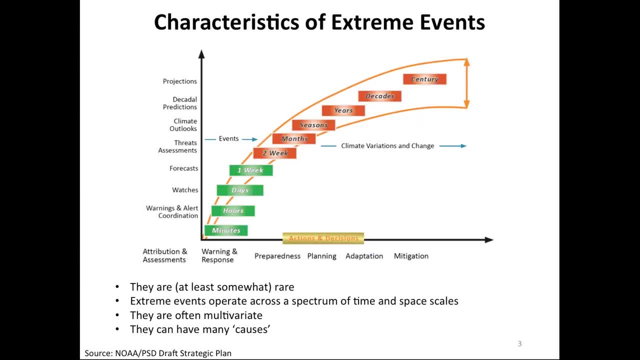 There's, you know, a range, but to some extent, extreme events are rare, which, as we'll see, poses challenges when we start to look at trends and what may be behind them. So we need to design those trends. 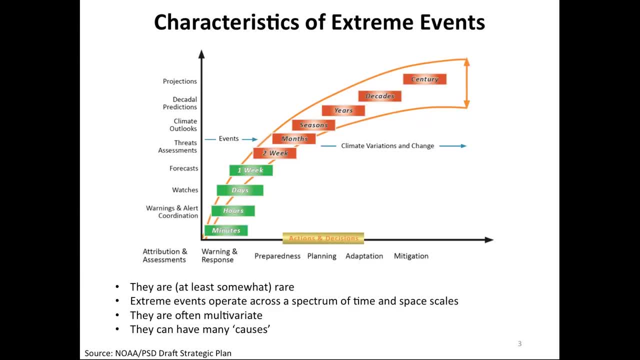 They're often multivariate, right? I mentioned the example of a drought before, But what exactly is a drought? I mean, most superficially, it's an absence of precipitation. right, That's how we're used to thinking about it. 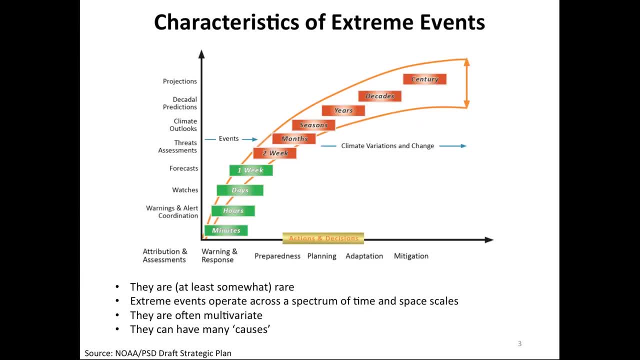 But of course we know that the higher the temperatures are, the easier it tends to be for soil, moisture or vegetation to dry out, right, So really we need to include consideration of temperature in any definition of drought. So things like you know how much water people are actually using. 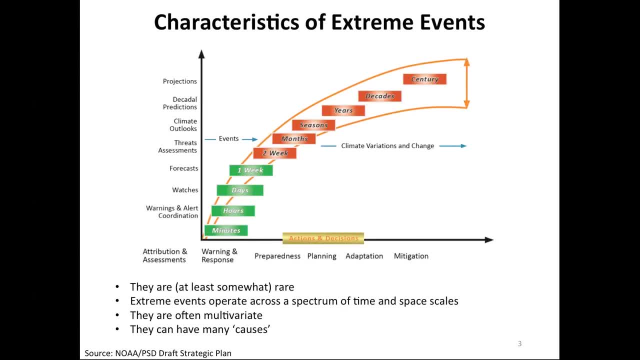 That's a dimension of drought too. So once we really start to unpack what an extreme event is this, multivariate nature can make it challenging, And there can be many causes that, in many cases, go beyond the meteorology and climate aspects. 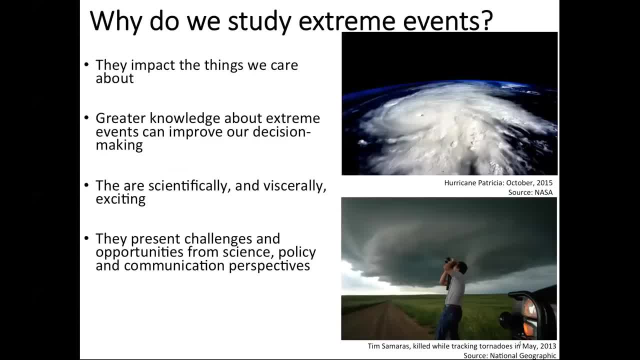 that we're going to be talking about. Okay, next slide. You know, really obvious, but I think you know an important reminder. You know my understanding is that a lot of you do on a daily basis. I know that this speaks very close to your experience and people. you know. 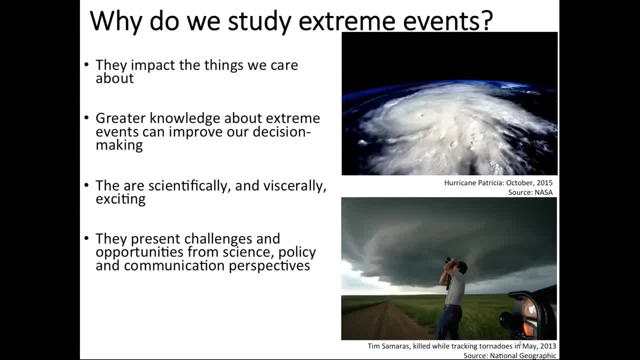 Obviously, extreme events have disproportionate impacts on the things we care about. whether it's Hurricane, Sandy, extreme heat events, People are vulnerable. Our ecosystems are vulnerable. Our infrastructure isn't always developed to withstand these kind of extremes, which leads to damage. 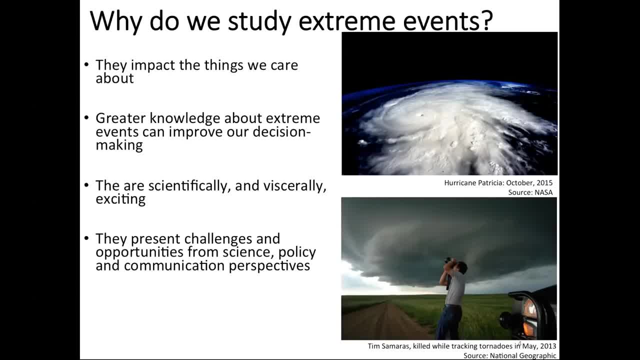 Also, you know the inability for certain missions and responsibilities to be met. Other reasons: we want to study extreme events. You know learning more can improve our decision making right If we can sort of delve in and think about utility grids. 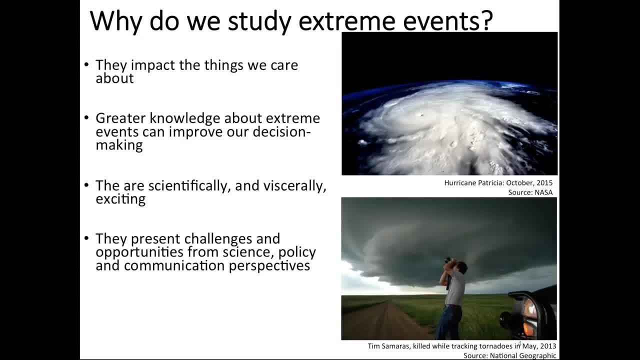 What are the temperature thresholds that are particularly important? for, you know, increasing the odds of power failures, for example. If we can study extreme events in a more deep way and link that to the knowledge of decision makers, there is really the potential to you know, that's one ingredient to improving a broad set of decisions. 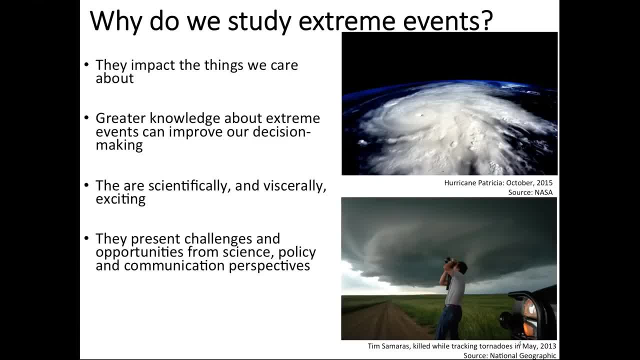 And I think it's important to be honest. you know from a scientific perspective, from a personal perspective, that these incredibly dangerous and often tragic events do have a certain draw. You know that's part of the story for some people, more than others. 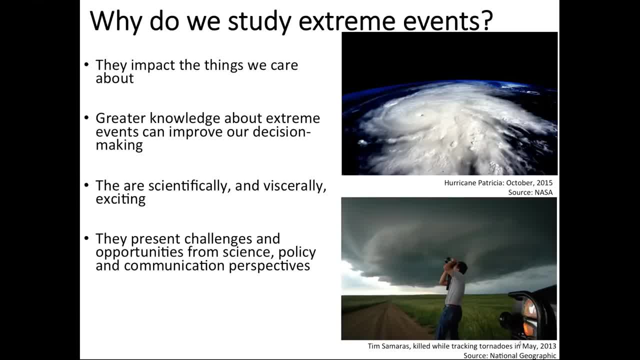 And there are opportunities. And there are opportunities to engage the public and engage communities in thinking about these kind of extreme events, And certainly they present challenges but also opportunities from science, policy and communication perspectives, Whether it's a public that's, you know, sort of open to thinking about their vulnerabilities to extreme events after they hit. 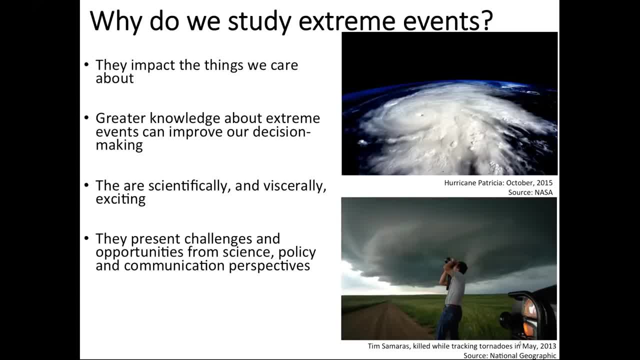 to leveraging, you know, people's willingness to sort of collaborate and help each other after certain types of extremes, To maybe opportunities to rebuild in different ways after catastrophic events, and leverage funding opportunities to increase our resilience. These are all things that can be thought of, you know, particularly, but not exclusively, through the lens of extreme events. 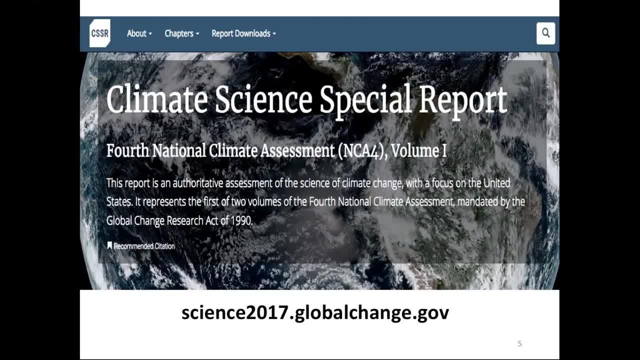 Okay. So, as Sean, you know graciously mentioned, I've had the good fortune to contribute to national climate assessment the third time around, And then this climate science special. This climate science special report was essentially part one of the fourth national climate assessment. 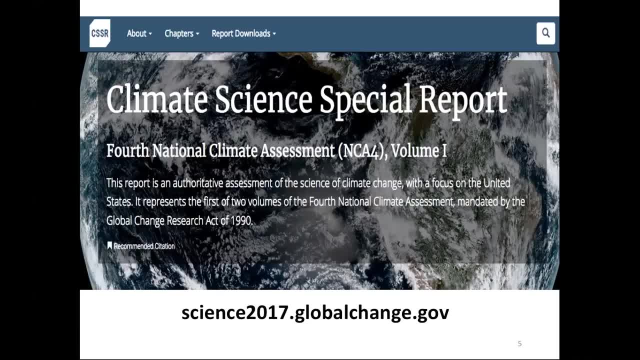 So a lot of what I'm going to show you today is historical trends in different types of extremes over the US that were produced by the diverse and rich author team as part of this climate science special report. So before we get into those specifics of extreme weather events and their trends, you know 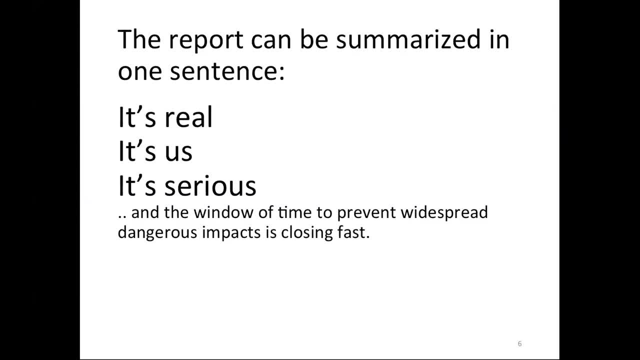 I wanted to highlight this one little statement that, in a way, captures so much of what's in this, you know, 600 page or more report. So climate change is real. Human activities are playing a critical role. It's serious. This is something that you know impacts all of us and it impacts all of us today. 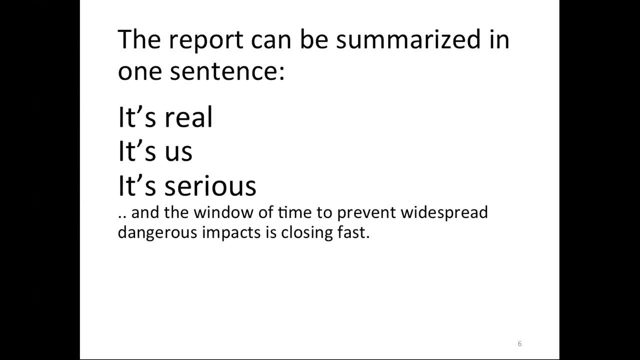 This isn't just a distant issue And we'll circle back towards the end to talk about the future, But I want to highlight the fact that the window of time is starting to close to prevent some of the most serious impacts of a change in climate. 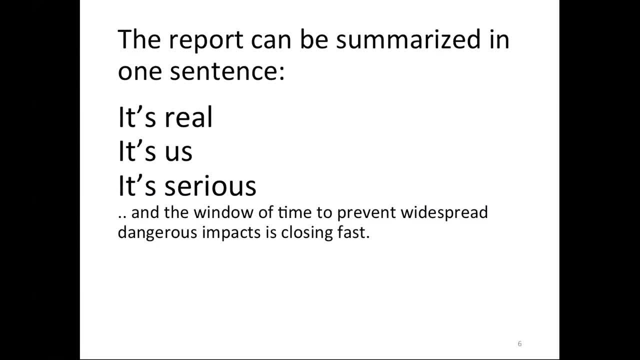 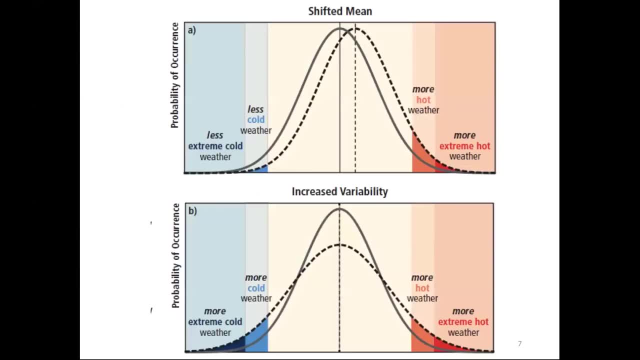 Some, but not all, of which are going to manifest themselves through changes in the statistics, the frequency, intensity and duration of extreme weather events. Okay, So now a schematic, just as we start to think about: how could the statistics of extreme events change in a change in climate. 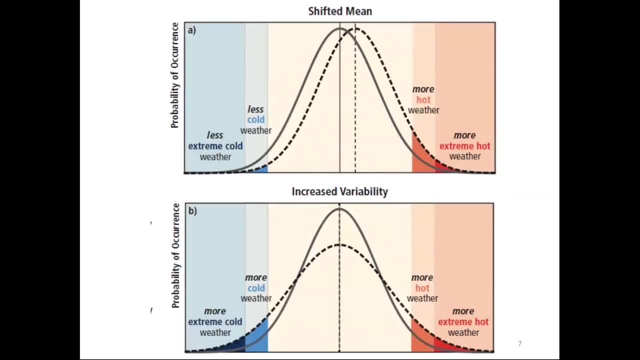 So if you look at the top figure here, you know, think of this as a histogram, Basically, for both of these figures on the X axis, you know, horizontally, you could have, you know, let's say these are temperatures. You know, really cold temperatures to the left, shown in blue. 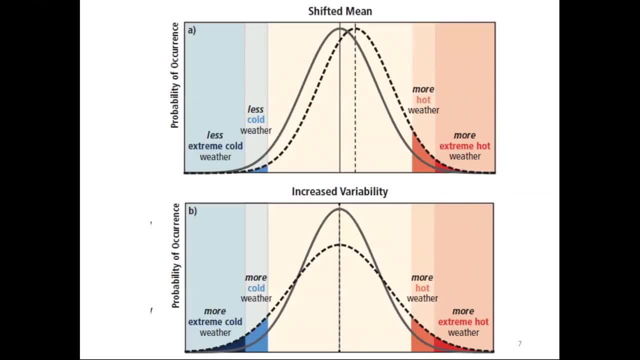 Really high temperatures to the right, shown with the red colors And then the Y axis probability of occurrence. So you know where I'm sitting in the lower Hudson Valley. you know you might have a high probability as shown in the solid. 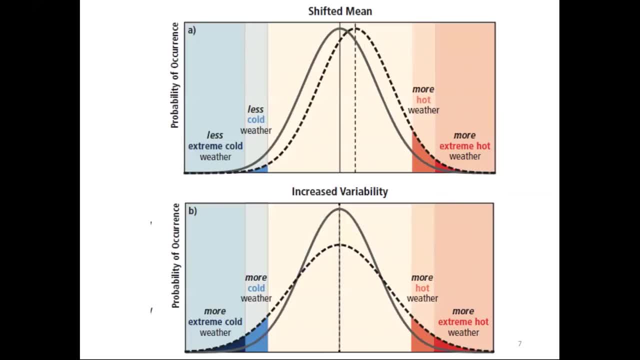 Okay, And then you have a solid gray line of temperatures. you know daily mean temperatures somewhere between 48 and 60 Fahrenheit. You know that's, you know maybe our most common mean temperatures. Not impossible for us to get us a day where the mean temperature is below 15 Fahrenheit. 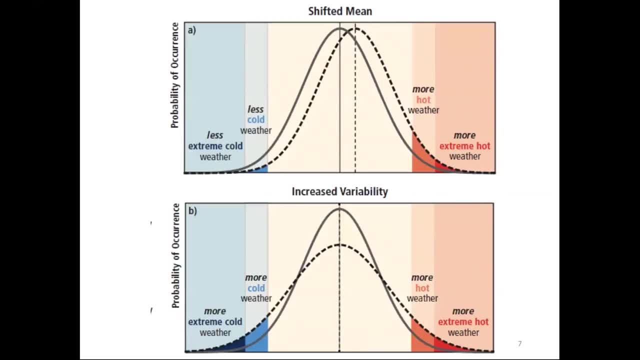 Also not impossible for us to get us a day where the mean temperature is above 92 or so Fahrenheit. So, even if we don't fundamentally change the nature of extreme weather events or not, the physical processes behind heat waves, just simply shifting the whole distribution, you know. 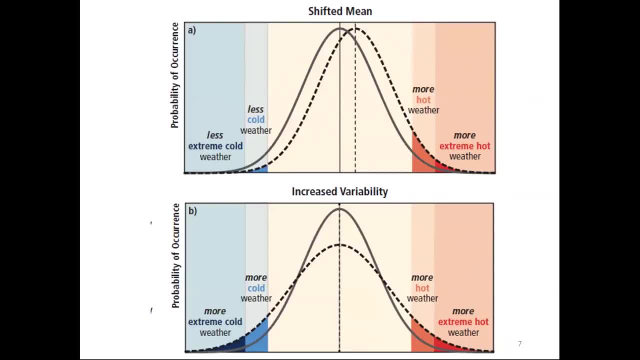 this mean global warming that we've heard about of you know- one degree or so over the past century, or the couple degrees that we're more or less locked into for the future, Even if the nature of individual heat waves- cold air outbreaks- doesn't shift at all. 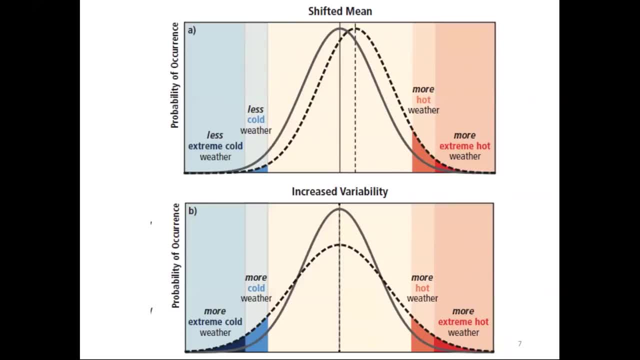 just maintaining that distribution pulls all the temperatures you know to the right, as you can see with this, with the dash line. So if we circle back to these temperatures between sort of 48 and 60 degrees again, I'm sort of focused on the top panel here. 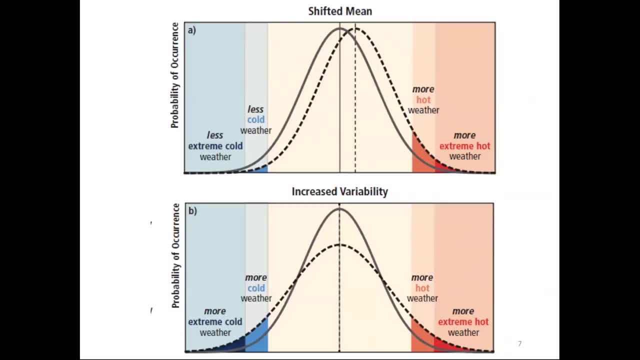 You see, from a you know, the probability of occurrence stays about the same for those, for those days around the middle of the distribution, those really common temperatures- Maybe a couple percent, you know- decrease in frequency of one at the lower end. 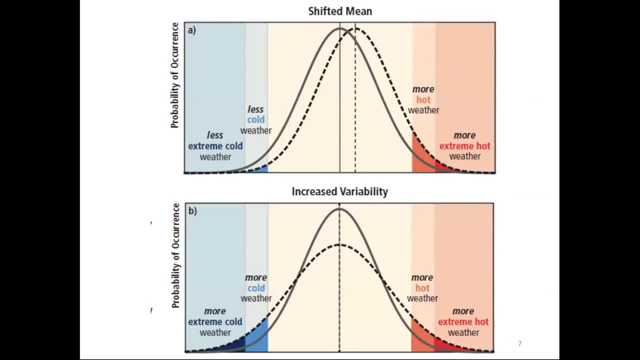 and a couple percent increase at the higher end between, say, 48 and 60 Fahrenheit. But if we look out at those tails where we see the biggest impacts right, a dramatic decrease in the frequency of really really cold events. We had a paper this past year that looked at a southern pine beetle. 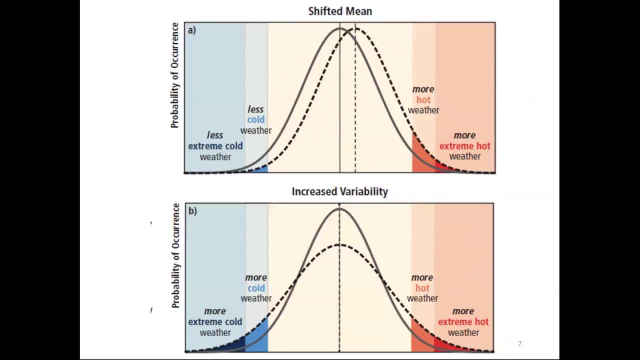 you know, key agriculture, key forest pests, ecological pests, that's highly sensitive to really cold temperatures. If you're not getting those really cold temperatures it's one factor that helps that pest to thrive And you can see small shift in average conditions gives you a large change. 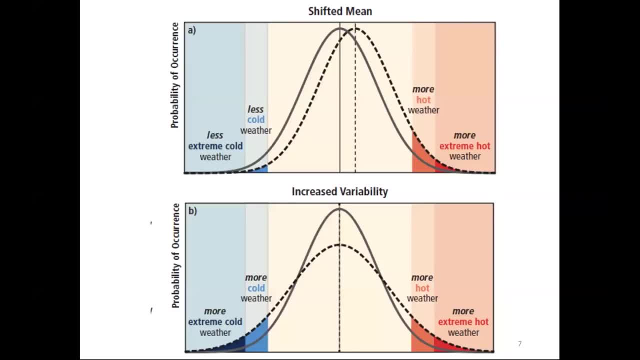 in the frequency of really cold days. At the other end of the spectrum, we're thinking about days for New York, you know, above 95, where the max temperature is above 95 or 100, that couple degrees of warming which doesn't sound like much. 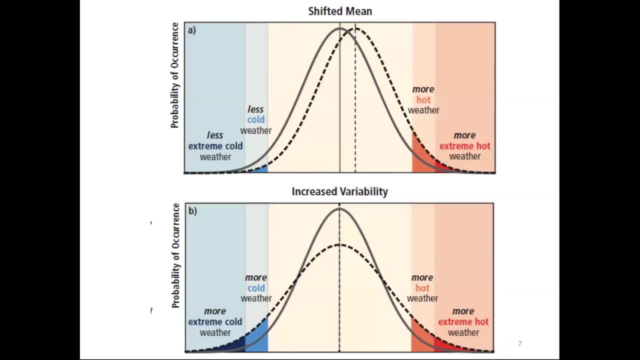 could double the frequency with which we're getting, say, 100 degree days. And of course it's not just the frequency of those days, it's the duration of the heat waves. right, We're talking about warmer nights, longer duration to those events. 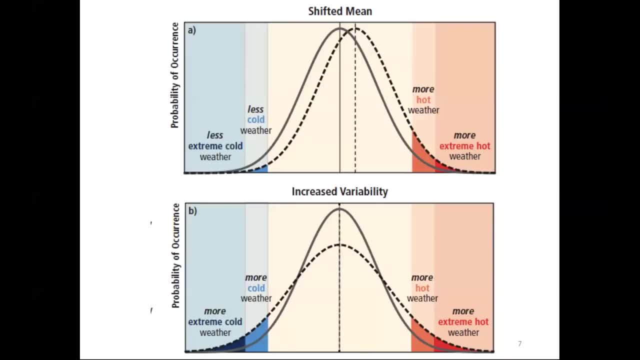 and higher absolute temperatures During them, you know, by a couple degrees doesn't sound like much, but it really matters if you're talking about 104 Fahrenheit instead of 102. That implies a lot of extra demand on the electrical system. 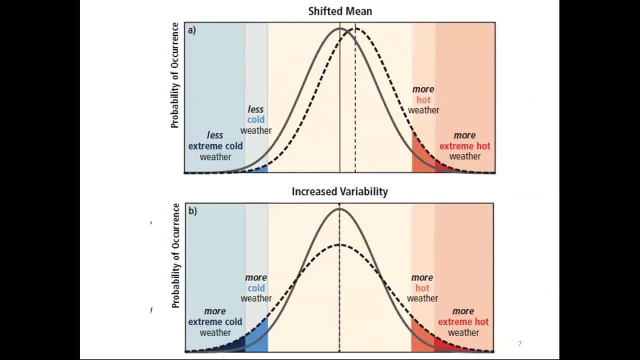 And we know that human populations are really sensitive. you know there's a nonlinear relationship as you get out on those tails those really, really hot days. So, point of the top figure, small shift in average conditions loads the dice and can have a big impact on the frequency of those days. 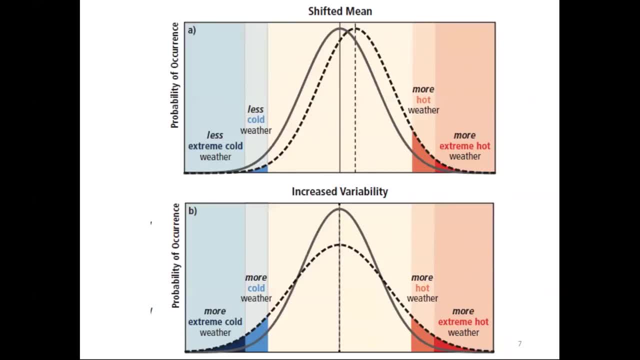 And that's one of these extremes that matters so much. But of course that's sort of the first order interpretation of climate change. You know, we also have to think about how might the actual processes themselves change. Maybe heat waves will change in some surprising ways. 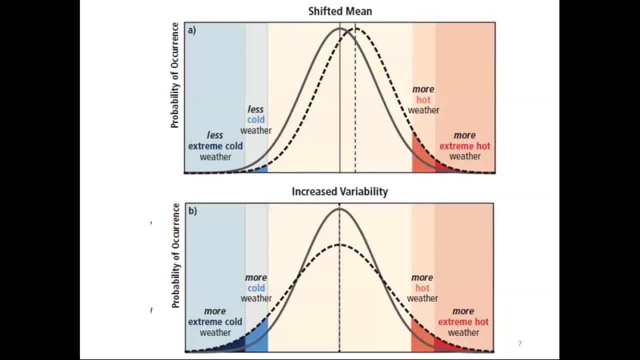 Maybe there will be feedbacks between loss of soil moisture as temperatures go up that thereby makes it easier for you to get more warming. since you know more sensible heat, less latent heat, Maybe the jet stream is going to change in the future in ways that will change. 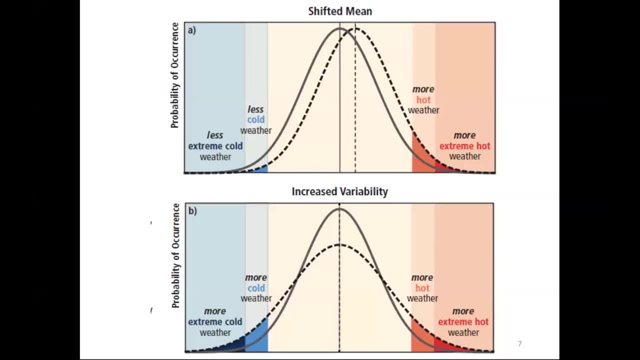 how often we get the blocking high pressure systems associated with heat, how long those tend to last when they occur, Or at the other end of the spectrum, maybe they'll, you know, change how often we get low pressure systems, you know. 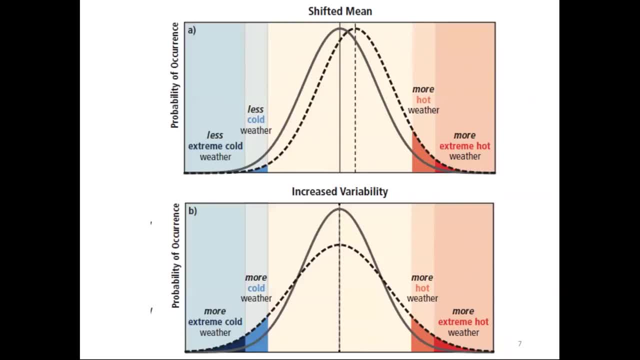 moving through some areas in the mid-latitudes during summer which, all things being equal, can cool us down through cloudiness, moisture, tendency to advect there, To advect there. out of the north, you know at least part of their passage. 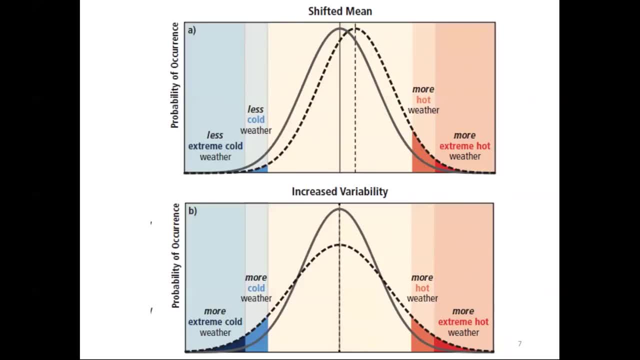 So the nature of extremes could change as well, And that's depicted in the bottom plot here, shown as an increase in variability that has a big impact out of the tails. But we also need to be mindful that, you know, there's more uncertainty about how these event processes could change. 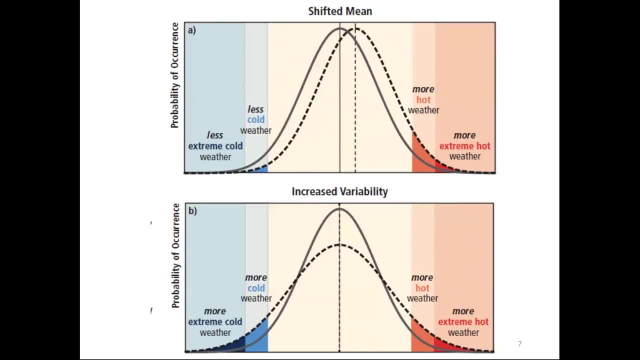 than there is about how the mean could shift. So it's not always going to be an increase in variability. That's going to depend on the variables, It's going to depend on the temperature itself. So bottom line of the top part of the figure, 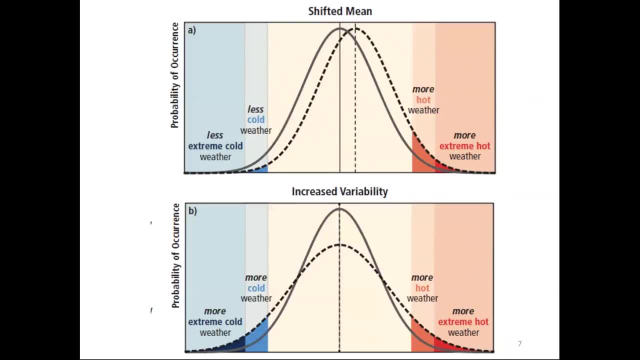 small shift in average conditions can mean a huge change in the frequency and intensity and duration of extremes. And then the bottom picture is this nuance of the events themselves could change in nonlinear ways with climate change. So just to quickly think a little more about that. 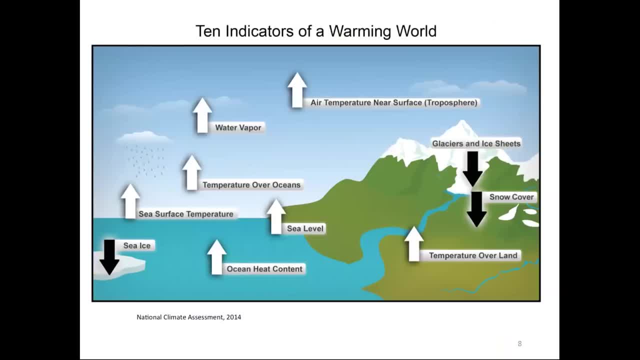 why might some of these processes change behind heat waves? Why might the statistics and the distribution change? But what we need to think about here is is that it's not just the temperatures are going up. The entire planet is changing. Storms, for example, that form today are forming in a different environment. 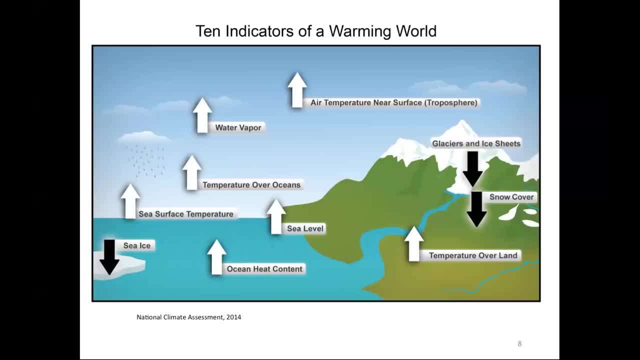 than they were when greenhouse gas concentrations were 40% lower than they are today, before the Industrial Revolution. We now have more water vapor in the air which, all things being equal- you know, if the dynamics stay the same- give us a chance for much heavier rain events. 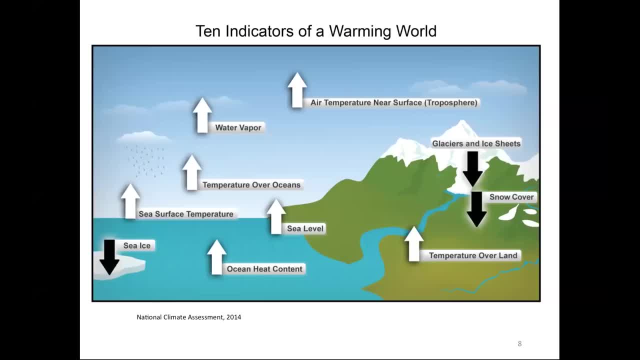 We have warmer ocean temperatures which again, other things being equal, you know, argue for stronger hurricanes, at least that the strongest storms might become stronger. Changes in the sea- ice could potentially impact the jet stream. That's an active area of research. 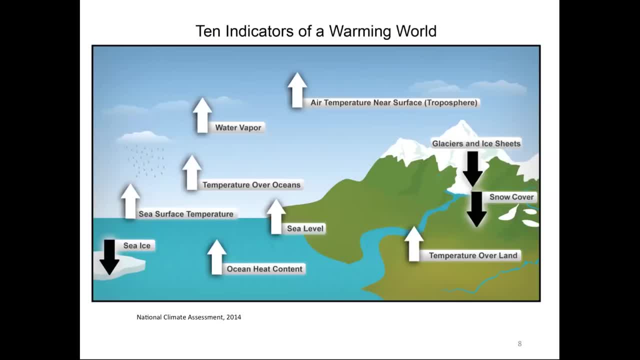 So just to sort of show that you know the ingredients, the sort of baseline situation is changing When any storm forms or any extreme event forms. it's a slightly different background than it was in the past. So those are really active areas of research. 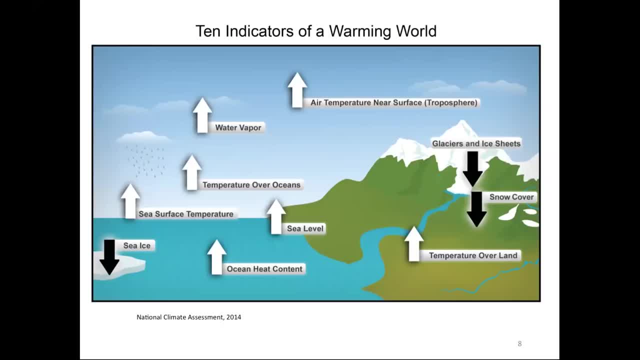 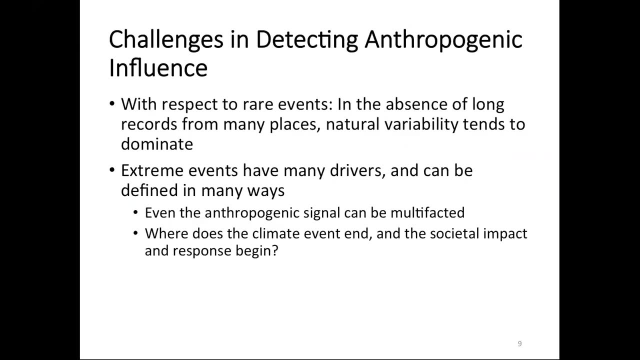 How these things may all interplay to impact extreme events in the future. So as we're now about to sort of jump into a study of trends and different types of extreme events, you know I do want to first again just sort of acknowledge some of the challenges here. 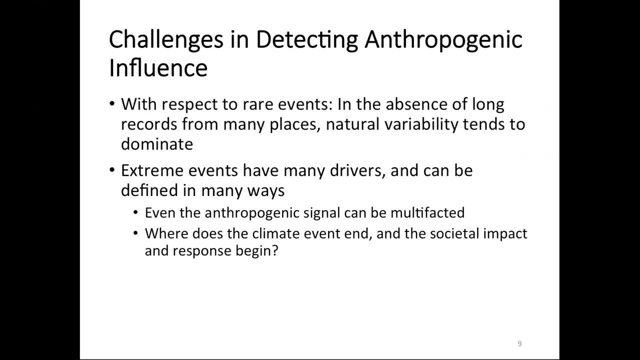 Some types of extreme events are really really rare, right, If we're trying to say in a particular place, what's going to happen to the one in 100 year drought event, the event that on average happens, you know, once every 100 years. 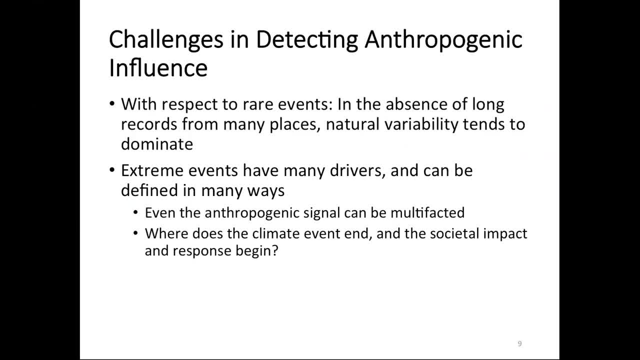 or the coastal flooding event that happens once every 100 years For any one place. when events are really rare, it can be hard to characterize the true baseline variability. before we even think about climate change, We can think about it, the sort of noise of variability. 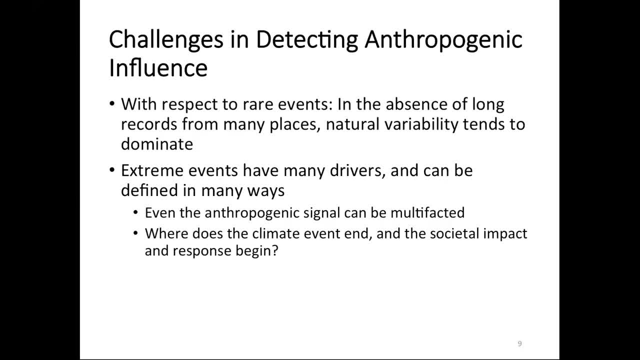 can be large relative to a climate change signal, even if a climate change signal exists. So you tend to need aggregation across a lot of states and a long duration of data set for some types of climate extremes in order to see any signal, if there is one associated with greenhouse gas concentrations. 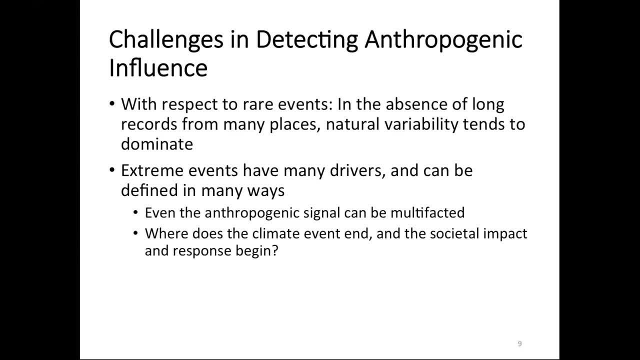 amidst the natural variability of small sample sizes, essentially So another thing that I alluded to earlier: when we think about an extreme event, you know it has so many drivers it can be difficult to unpack exactly what we mean. So if you hear people say, for example, that you know 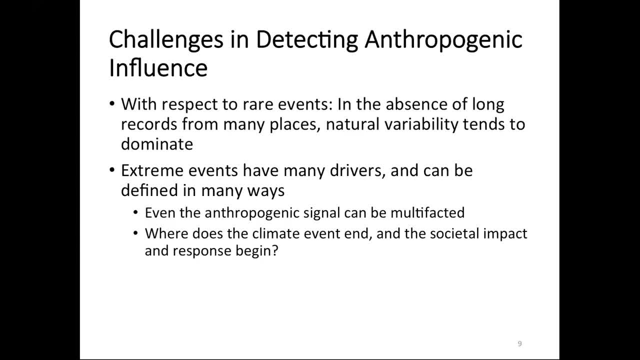 Hurricane Sandy was so Superstorm Sandy so devastating for the Northeast, possibly with a climate change link. What exactly are they talking about? Are they talking about the central pressure? Are they talking about the fact that it made this sort of left hook turn? 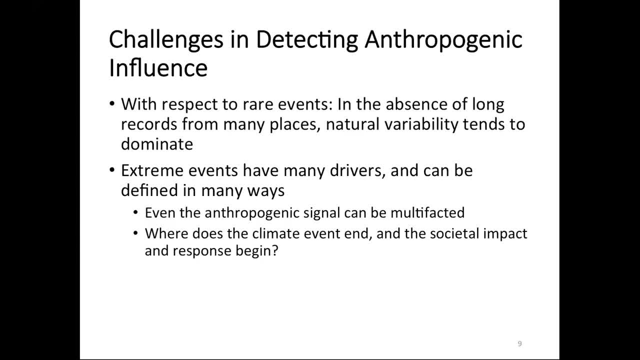 Are they talking about how high the water levels got, which is partly a function of sea level, partly a function of the fact that it hit parts of New York City at high tide? Unpacking exactly what we mean is important. Some aspects may have stronger climate change signals. 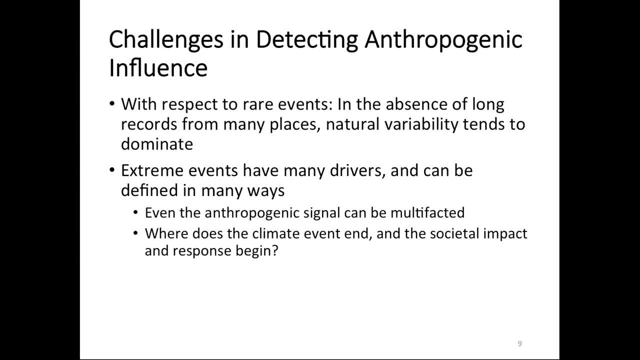 Some may be essentially random. So that's a key element. And when we talk about an extreme event, where exactly does the meteorology end And where do we get into societal impacts and human response? Thinking about Harvey, for example, you know their precipitation was so exceptional. 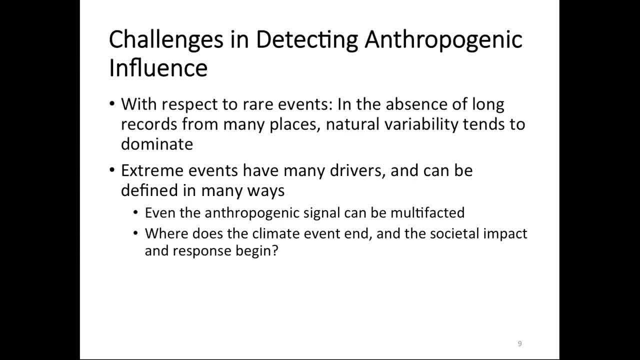 But where? when we look at the actual flood damage on the ground, how much is the heavy rain, How much is land use decisions that have been made that you know remove the ability to capture some of that water? Clearly there's a little bit of both. 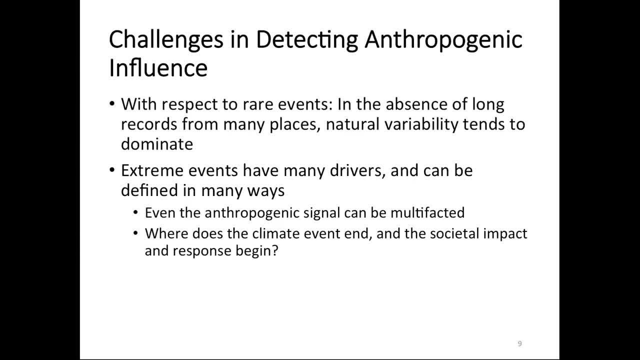 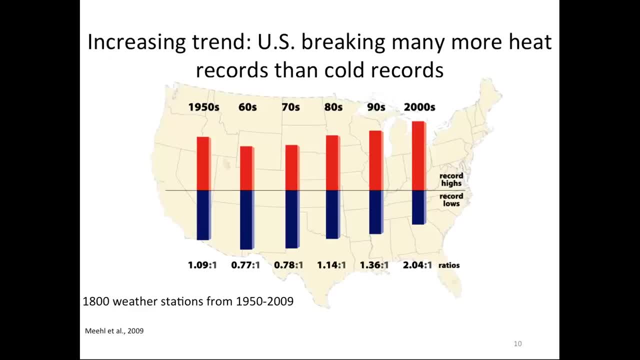 There's a lot of both, Unpacking exactly what we mean when we talk about a flood. you know how much is the meteorology, How much is climate change. It's challenging, Okay, So now let's jump into some actual data here. 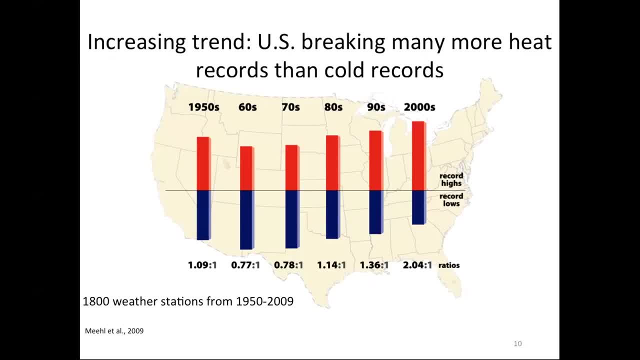 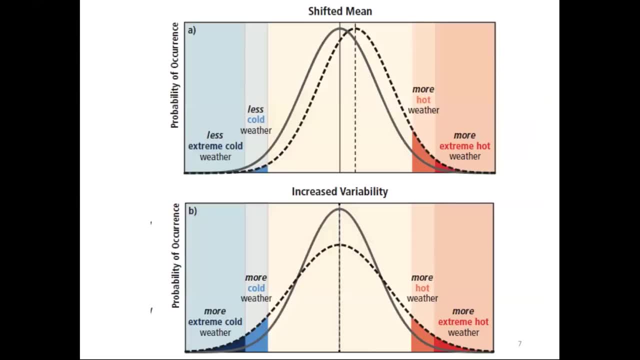 So I'm going to start out talking about temperature extremes. So circling back, just to remind everyone in this top panel here, if you just shift the mean, we'd expect to see potentially pretty big changes in the frequency of record-breaking high extremes increasing. 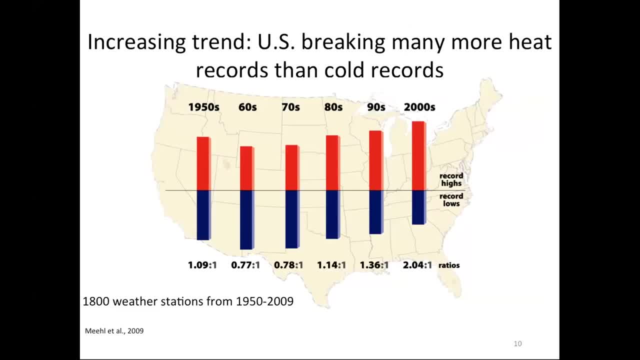 record-breaking low extremes decreasing. And indeed, when we go, look decade by decade, across 1,800 weather stations in the US, showing here the ratio record-breaking high temperatures to record-breaking low temperatures for each calendar day here. So a record-breaking high temperature can happen in January. 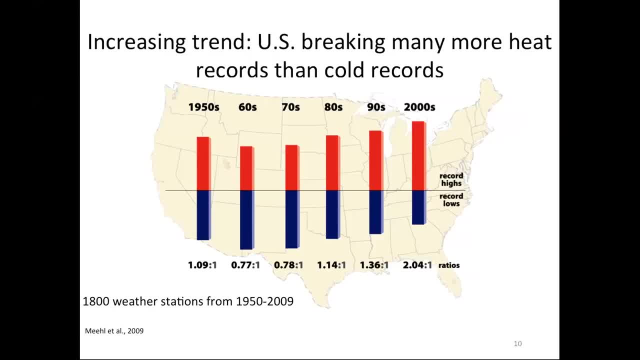 record-breaking low temperature can happen in July. This is just, you know. for each day You can see a ratio close to one to one for most of these decades, Periods actually, where there were more record-breaking cold than warm. Some of that might be natural variability. 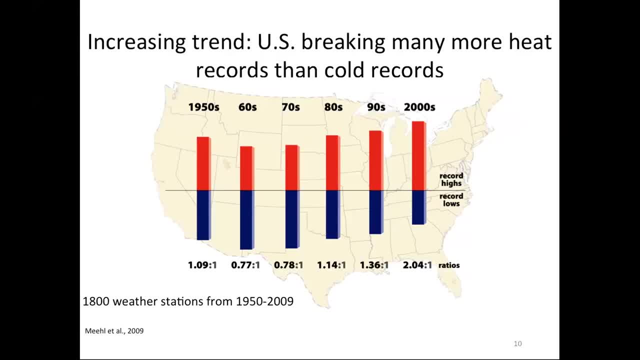 Some of that might be the impact of aerosols that block sunlight, But what you can really see here as we move towards the 2000s is, with really just essentially about one degree of global warming, we'd already reached a state where you had more than twice as many record-breaking high extremes as low. 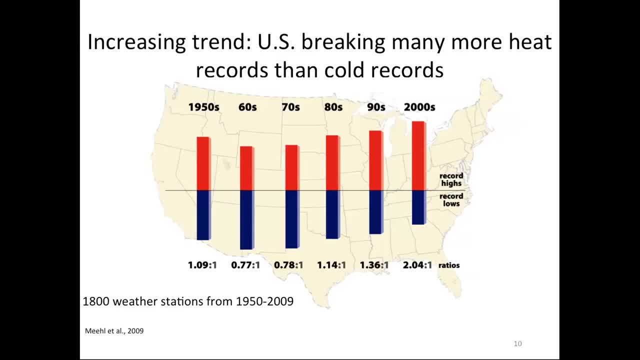 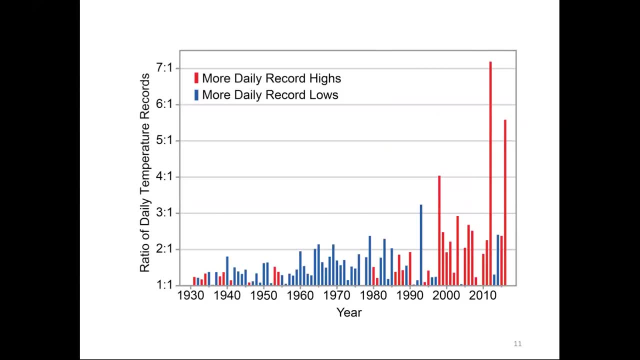 extremes with just one degree or so of warming. And if we look year by year, going back actually to an earlier period, you know a few things jump out. So this is the ratio, You know, if there's more cold than warm extremes. 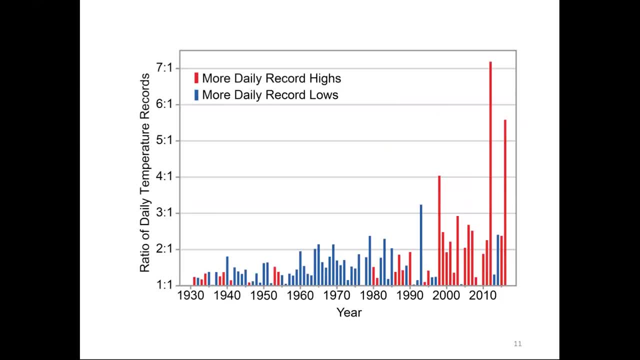 you get the blue color, More warm than cold, you get the red color. So you can see, you know there's year to year variability And during this last decade there have been times over the US as a whole where you 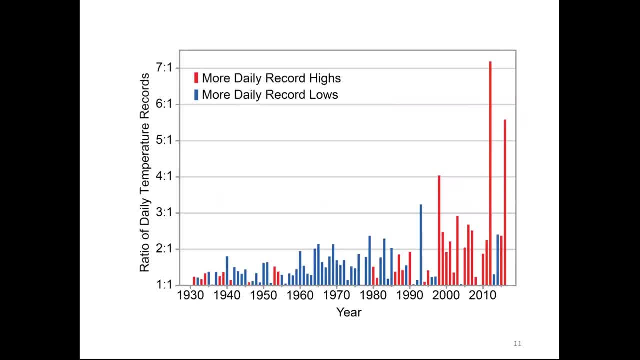 you know, if you look at, I think that was 2014,. more than twice as many record-breaking cold extremes as warm. There's still some variability there, even if we average across the US, But a signal is clearly emerging If we're thinking about building the infrastructure for the future. 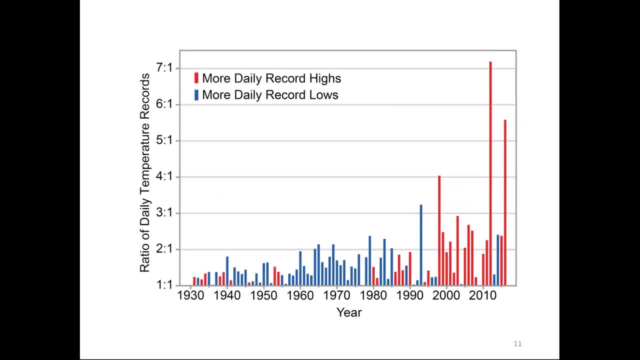 you know, protecting population from dangerous heat in the future. you can't any longer, you know, plan for the climate extremes of the of the past, The long, long term, if we're thinking about 10 year plans, 30 year plans. 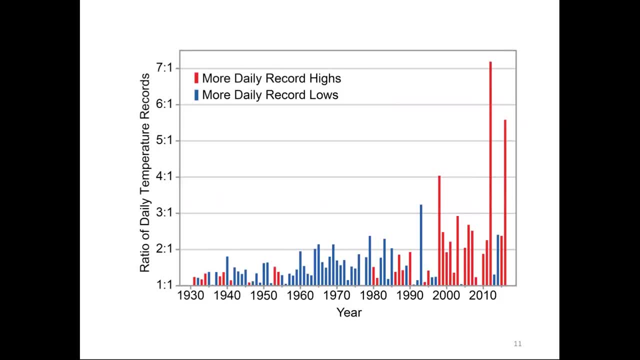 the statistics have clearly shifted. Now a lot of what you're seeing in this plot, you know some of it could be natural variability. I certainly don't mean to argue that this seven to one in the year 2012 is entirely a change in climate. 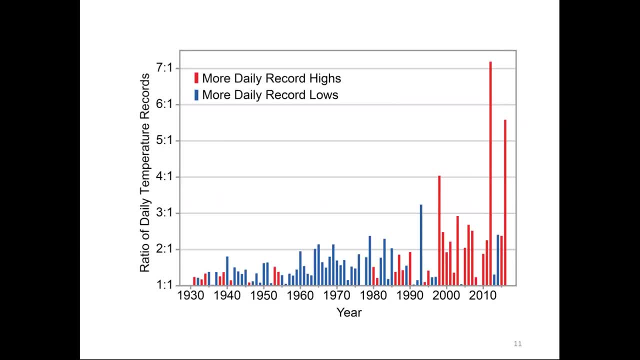 You know there's there's variability embedded in here, But a signal is clearly emerging And this is 1800 weather stations. You know it's going to be just you know sort of local effects you know which could be relevant in some places associated with. 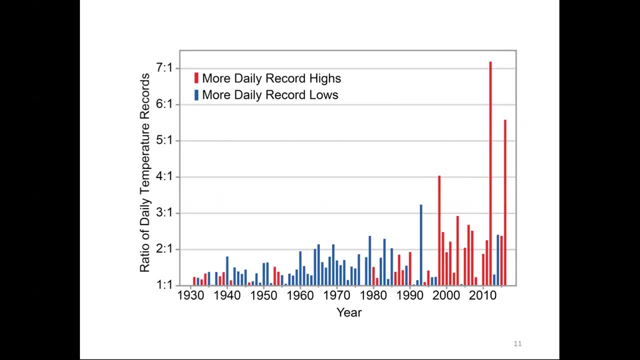 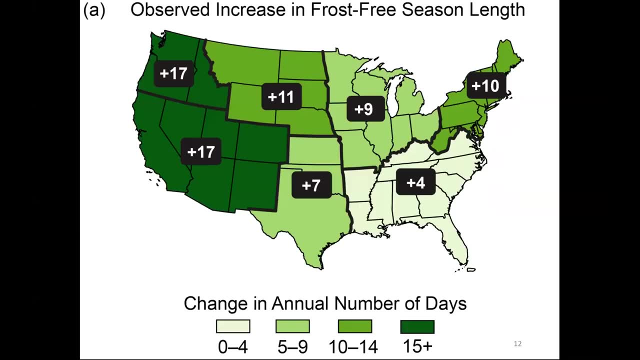 with the heat island, for example. This is- this is, you know, much broader phenomenon. It's also observed globally to some extent. Okay, So something that we might not immediately think of as an extreme event, but, but that sort of 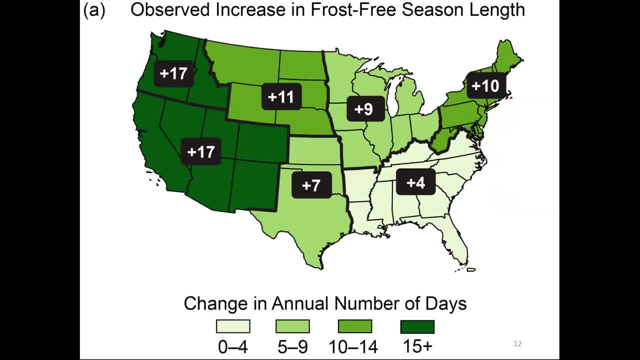 you know, reflects an integration, if you will, of extremes, The increase in the length of the frost free season, very robust trends across the US, particularly as that mean shifts upward, It's harder to get get freeze events, And so 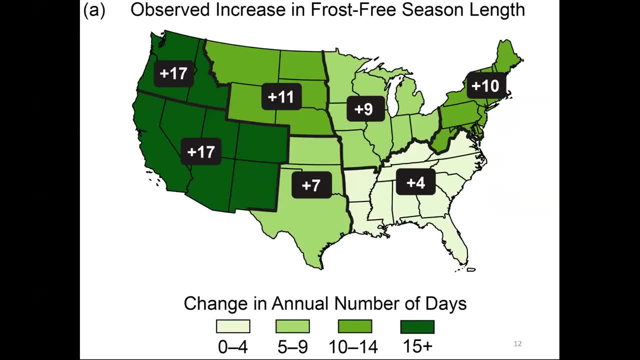 so. so the duration of that frost season going down pretty dramatically again, just with a little bit of global warming. so far already big shifts And some of these metrics that are critically important for society. Okay, Let's shift away from temperature. 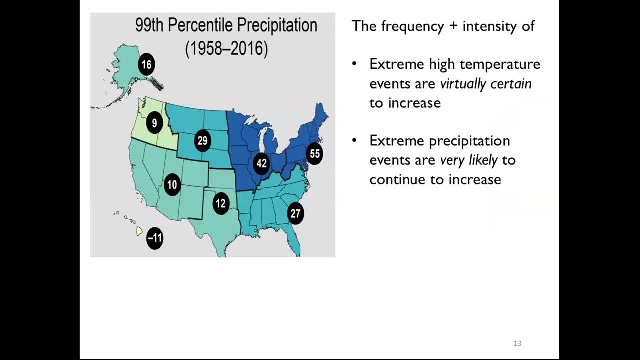 Now talk a little bit about extreme precipitation. If we're looking at, you know, annual average precipitation, most of the US trends have been pretty small and many cases haven't emerged at the annual scale from that natural variability that we talked about earlier. 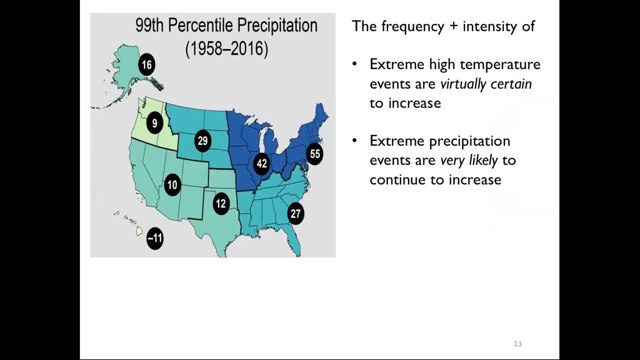 But if we look at the really heavy rain events which are, you know, often defined as, within the rainy days, the 1% rainiest of those days, that's a common definition. If we look at the amount of rain falling in those heavy rain days across the 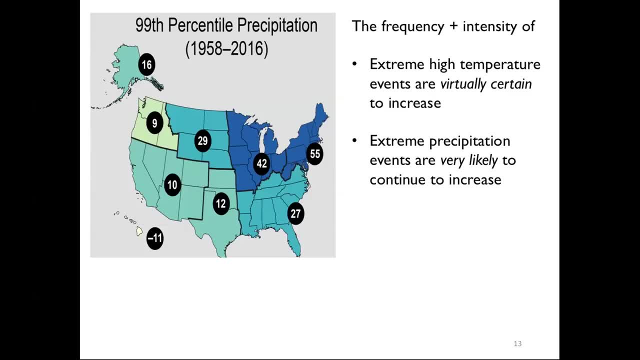 entire country, exception of of Hawaii, we're seeing those really heavy rain events either becoming more common or holding more rainfall leading to more rainfall. You can- you can define it either way and get pretty similar numbers. So across the Northeast. 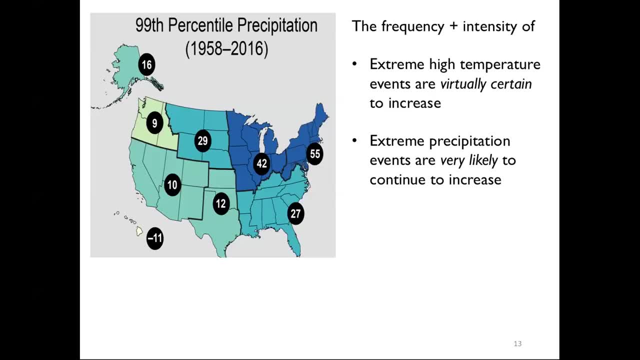 this trend you know has been, you know, 55% increase over about 50 years. And again, don't focus on that exact number. There's a lot of natural variability in here, but that's a powerful you know. 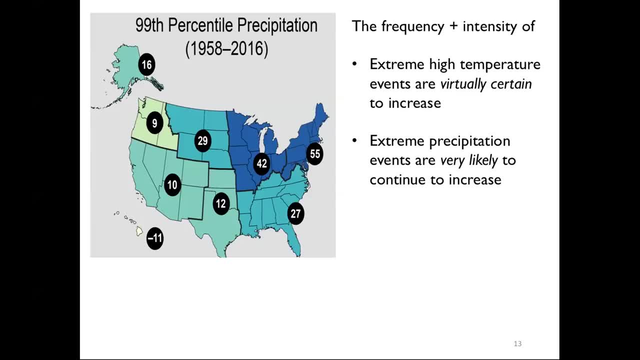 powerful change, And we see it over other parts of the world as well, And of course, it's consistent with our physical understanding of you. know why you should see heavier rain events as the atmosphere warms and can hold more moisture Now. 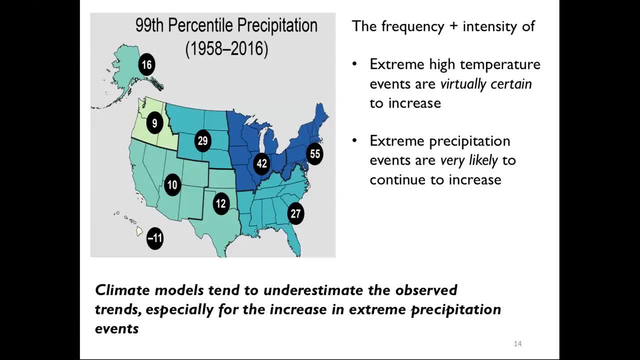 another important point here to mention is that climate models have limitations, and this can cut both ways from a risk management perspective, You know, if we really want to consider the full range of possible outcomes which can be so important. if we're, you know. 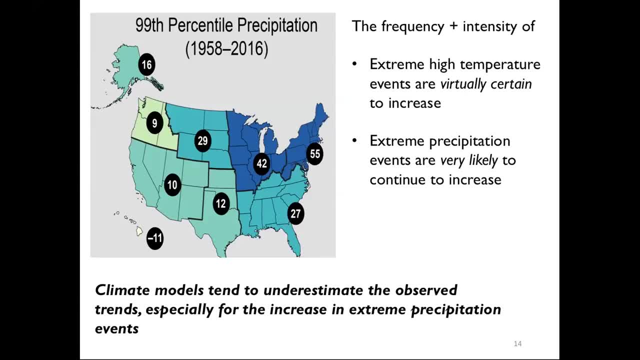 thinking about fail safe infrastructure, public safety. we need to be open to the idea that, you know, climate models may not capture the full range of things that can happen And for something like heavy rain, which often, especially the sort of 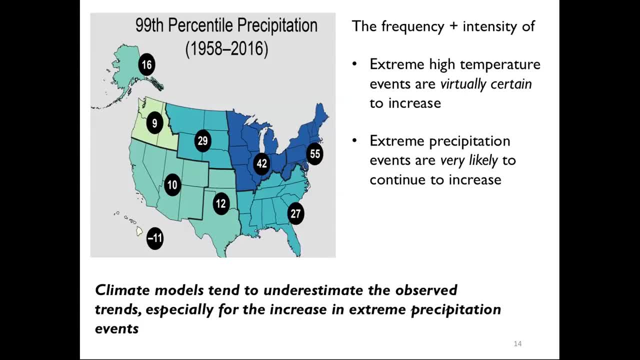 you know warm season convective, you know local types of events. climate models aren't really at the right spatial resolution to capture everything that can happen there, Certainly when we look at what happens when you run climate models over this historical period. 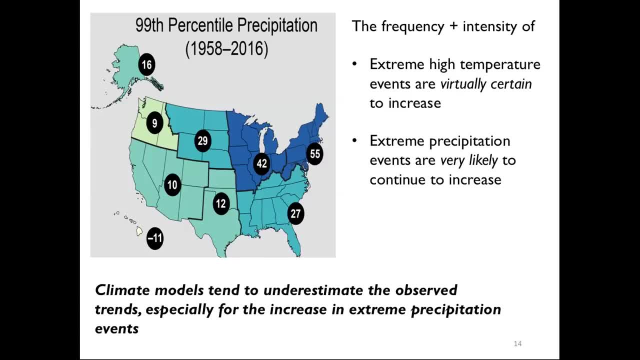 with the greenhouse gas concentrations that were present, you know, sort of increasing as it did over the last 50 years. climate models will show an upward trend in extreme precipitation but they can't capture these very fast trends, these fast increases. So it's more likely than not that the climate model results would underestimate. 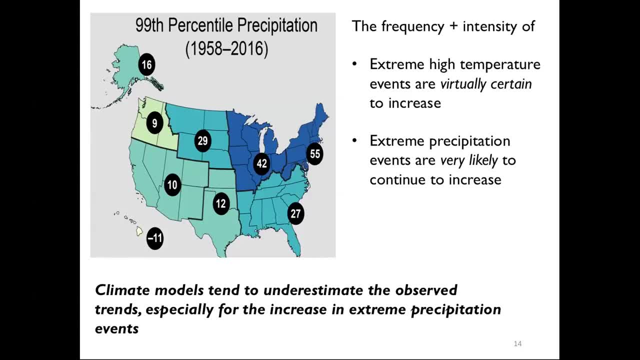 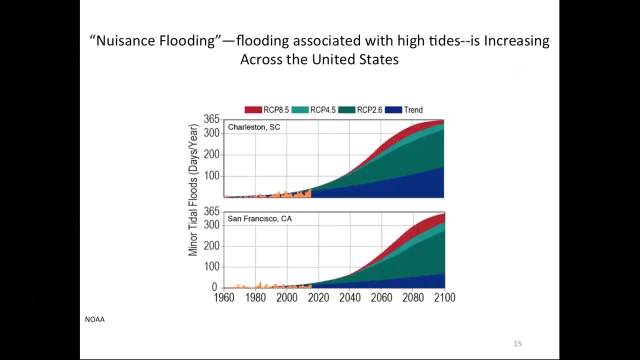 if we relied just on models, how much heavy rain events could change in the future? Okay, so now let's shift gears to a different type of flooding. This is a really important plot showing how the frequency of coastal flooding is affected by these small shifts in average sea level. 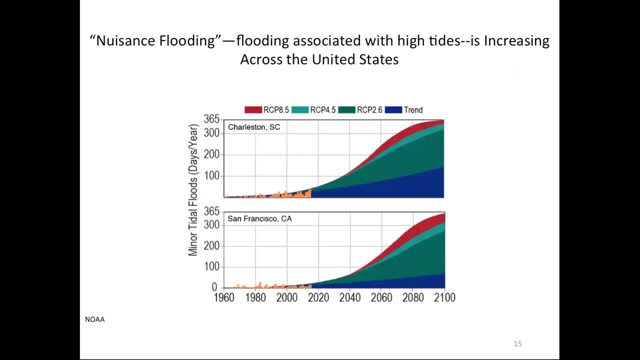 We hear about, you know, seven or eight inches of global sea level rise over the last century Sounds like nothing. How could that matter, right? Tidal cycle in a lot of places is four feet or more in many places. How could seven or eight inches of sea level really matter? 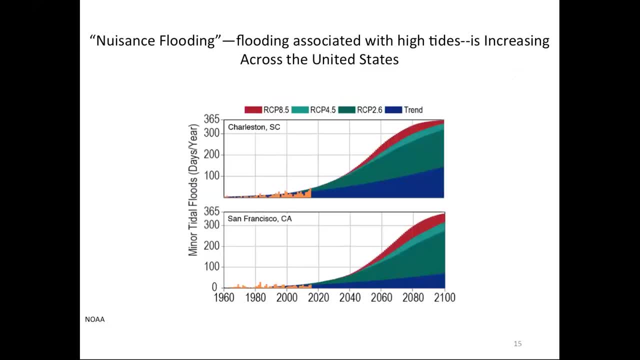 Well, of course they matter because they're present all the time. It raises the baseline, it raises the floor, it's making it much more easy to get high water levels of a certain height. You know the cliche I always use is: sea level raises the floor of the basketball court. 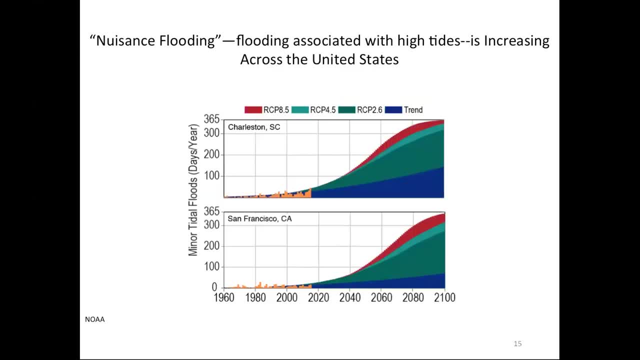 You know, and if a slam dunk is, you know, at 10 feet on that rim there aren't that many people who can slam dunk at 10 feet. But if you raise that floor just eight inches or so, it's not just a little bit more people who can dunk. 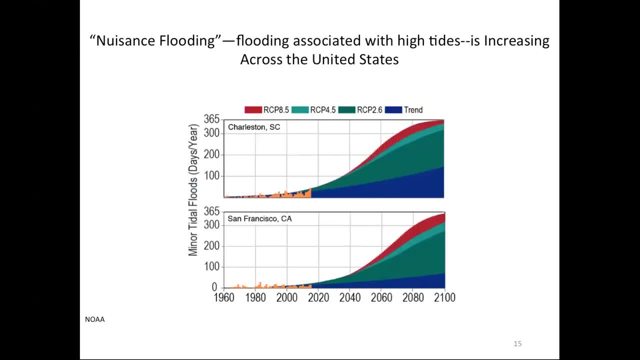 it's a lot more. So you dramatically change the frequency of coastal flooding With a small shift in that baseline. So, looking again, focusing on the historical part here, not projections for two cities along the coast with long-term tide gauges- Charleston- 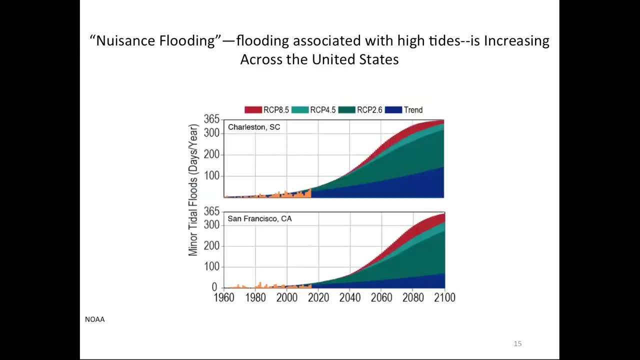 San Francisco very different environments. You can see that this nuisance- flooding the kind of thing that happens maybe a few times per year at the baseline sea levels of 50 years ago- a nuisance, when it happens, hard for some people who live right along the 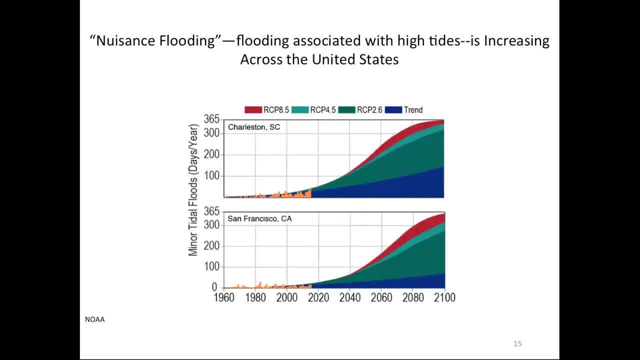 coast to get home from work. a little bit of water maybe in a few people's basements, in some people's basements. not necessarily a life changer if it's only happening a few times a year, but you can see already that yellow line, that for many of these places 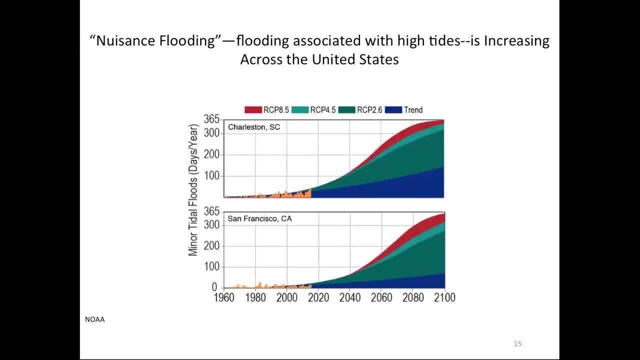 especially Charleston, already having maybe something on the order of 30 or more of these events per year, as opposed to a six. that amount perhaps 40 or 50 years ago, you know, with just with those small amounts of sea level rise. 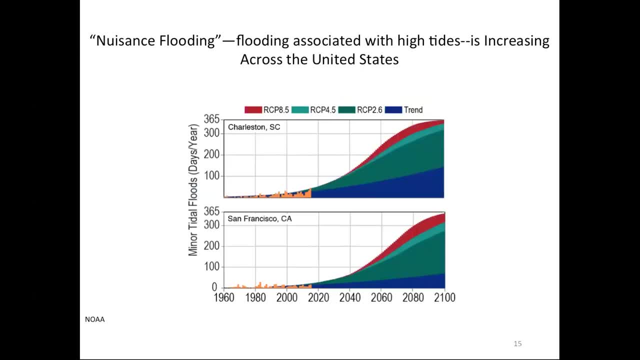 Charleston's actually had a little more sea level rise in seven or eight inches, but that's. that's not central to this story. You can- you can see the same patterns in San Francisco, and we're not going to talk a lot about projections. 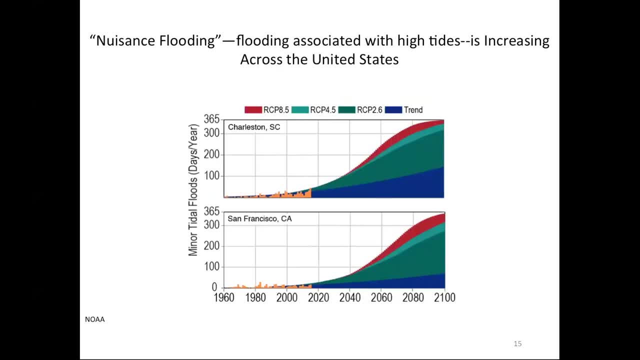 but you can see you don't have to go to extreme sea level rise scenarios. The historical trend continuing in sea level really gives you a transformative risk in terms of how often these events happen in the future. That's the nuisance: flooding. What about the biggies? 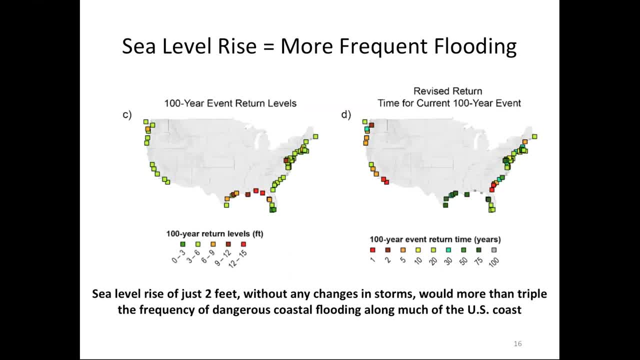 What about the more catastrophic flood events? So here now let's focus. I just got time to quickly look at each of these on the left for tide gauges along the US. What's the amount of high water? How big is the surge essentially associated with that? one in a hundred. 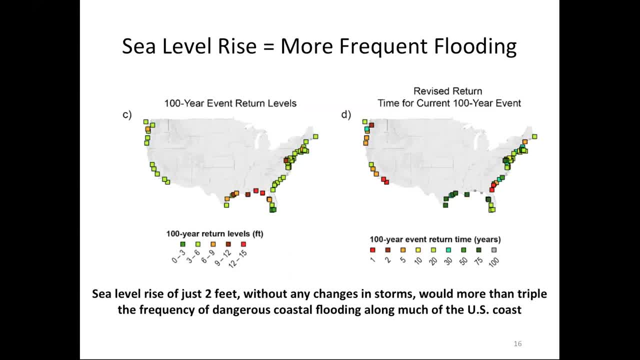 one, one in a hundred year event. So, as you'd expect, parts of the Gulf coast jump right out at you, right? No surprises there. Every hundred years we estimate. clearly there's uncertainties in these estimates. We don't have that long a record. 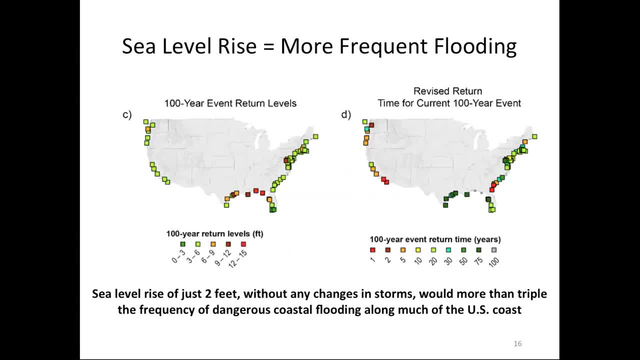 but on the order of 12, to 15 feet might be a one in a hundred year surge. Other parts of the coast, San Francisco, where you don't get huge, certainly don't get tropical cyclones very often, If ever the surges there might be more on the order of three to six feet. 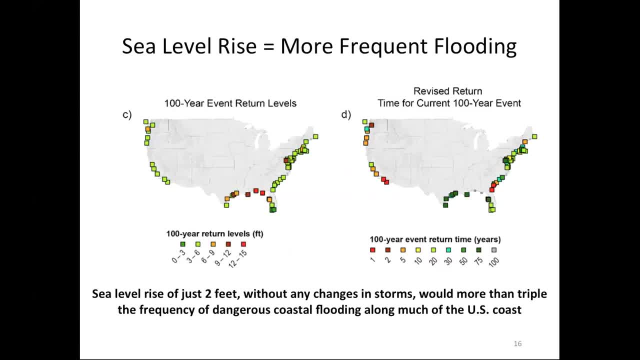 Now let's look at the right. The right is showing you with two feet of sea level rise, which is a conservative estimate. We'll be lucky if we only get two feet of sea level rise by two generations from now, for example by 2100.. 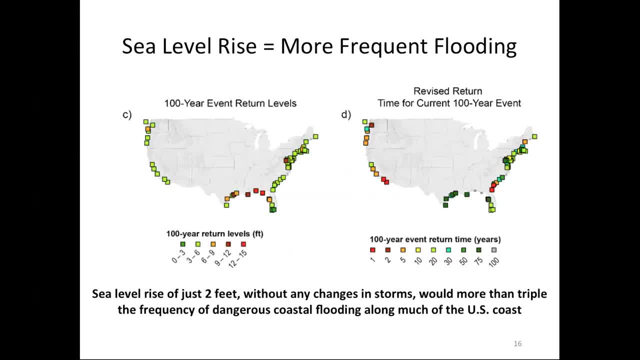 But even if we only get two feet of sea level rise and even if the nature of storms doesn't change at all- we're not invoking stronger hurricanes, We're not invoking changes in nor Easter's, just the storms of the past- That two feet of sea level rise presents a transformative change in. 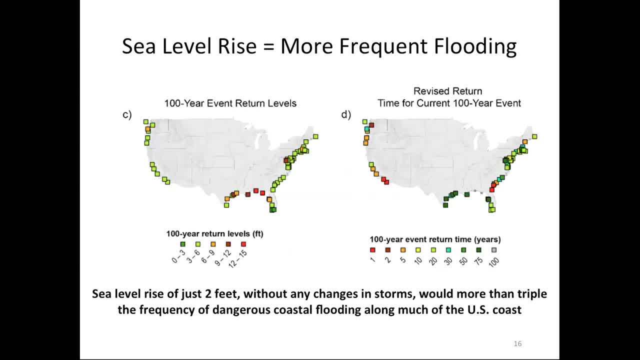 frequency right. So anywhere you see red there and the figure on the right that's places that historically had that high water level Once every hundred years. they're going to be experiencing it roughly once every century. They're going to be experiencing it roughly once every year. 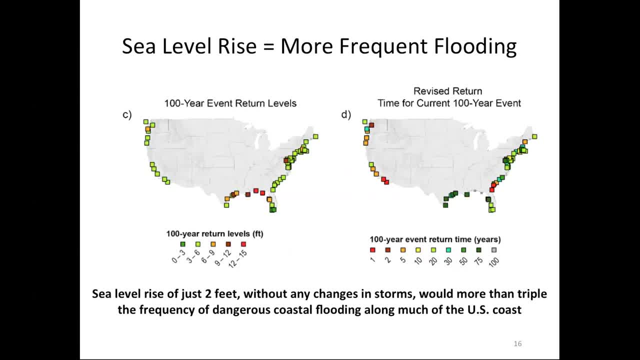 but just two feet of sea level rise and no change in storms. That's what raising that baseline, raising that floor does. You don't need stronger storms to get that catastrophic Flooding. And you see that all along the coast, even in the places that are relatively better off. 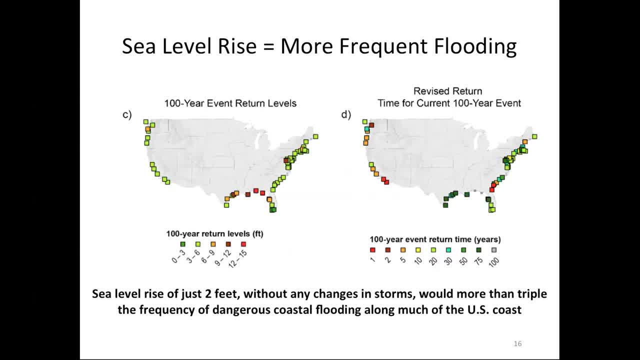 You know those light greens, even you know one turquoise in there. things that used to happen once every hundred years in terms of high water levels from storms- they're going to be more likely to cause more flooding than they used to. 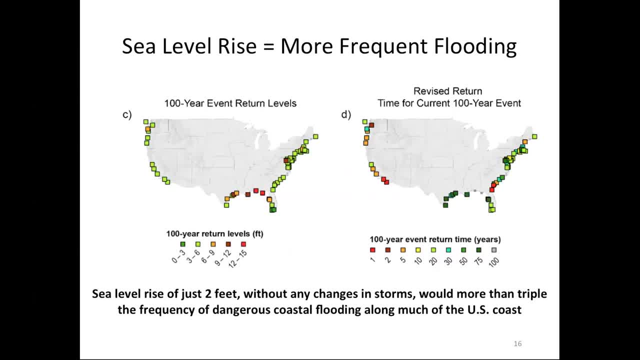 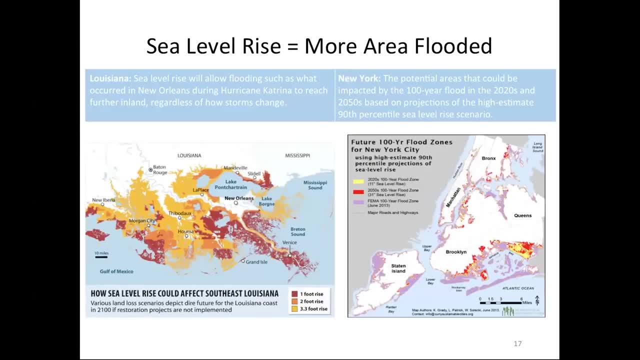 And so you can see that that's happening within the lifetime of the typical mortgage. So this is, you know, we're locked into this. two feet of sea level rise. This is a, you know, a fundamental challenge going forward, no matter what happens to storms themselves. 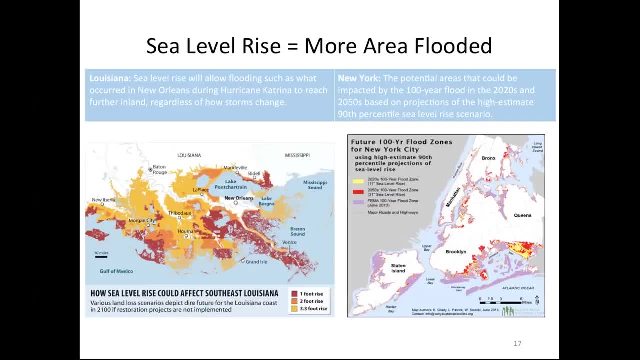 And that sea level rise doesn't just mean more frequent coastal flooding. What you're seeing here in these colors is how, for a given event, for a given storm, if you will raising that sea level, Means additional areas getting flooded that didn't in the past. 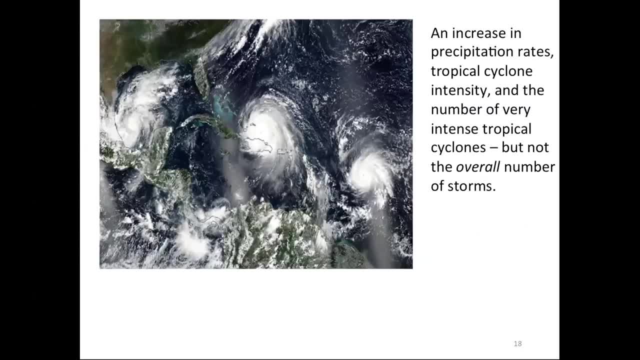 And so this is a this is a big, a big, big issue. that's going to be. that's going to be a big challenge for for for New York city. Okay, I want to keep us moving. I'm mindful of. 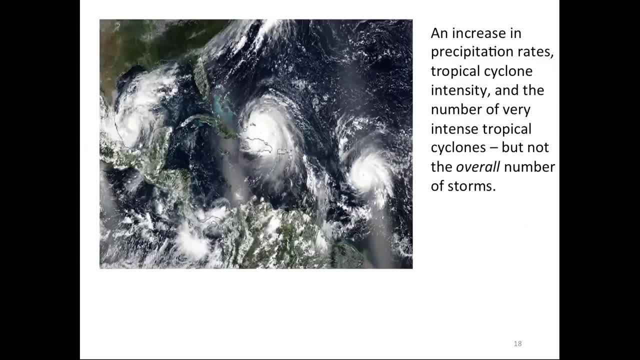 of time here. Let's quickly talk a little bit about some other types of extreme events. Certainly, everyone wants to know what's going to happen to Tropical cyclones. I think this is one of the more nuanced pictures There's, you know. 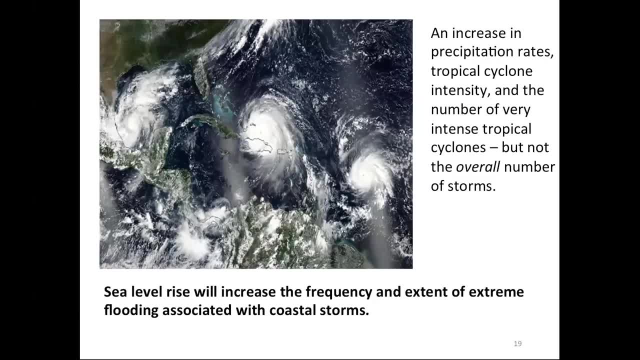 some things that we know more or less for sure. as I just said, sea level rise is going to increase the frequency and extent of that. as the atmosphere warms for a given hurricane of a given strength, there's going to be more precipitation associated with it. Some studies have: 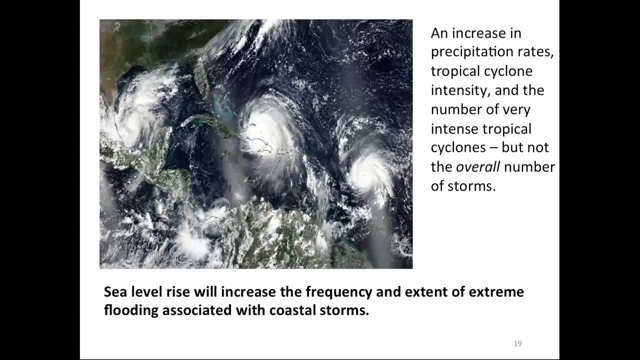 suggested, you know, maybe 10% increase in precipitation per degree Celsius of warming, But you know that'll also increase the risk. I think it's also certainly fair to say that the balance of evidence suggests that the major hurricanes- the category three, four and five- become more frequent and more. 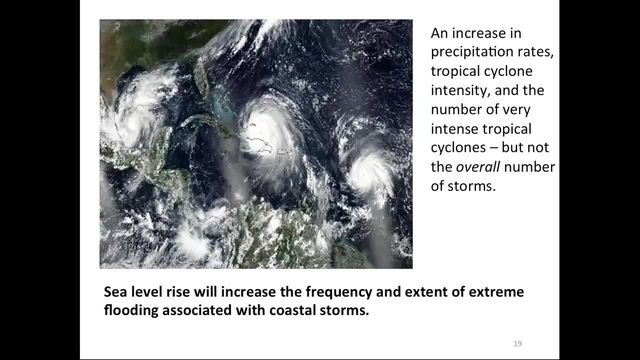 intense as the planet warms, largely because of their sensitivity to sea surface temperatures and the upper ocean temperatures, which we have high confidence are going to increase with climate change. Nevertheless, you know, I think that this is a case where we can't quite call this. 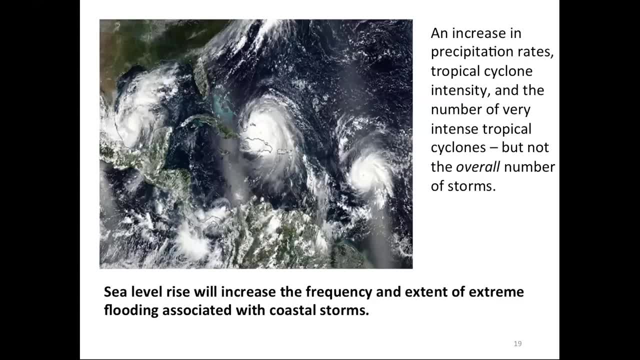 one a sure thing, And certainly if we're talking about tropical cyclones as a whole, tropical depressions, those storms that don't quite get to hurricane status, balance of evidence, you know, probably suggests, maybe, that the amounts stay about the same. I think we 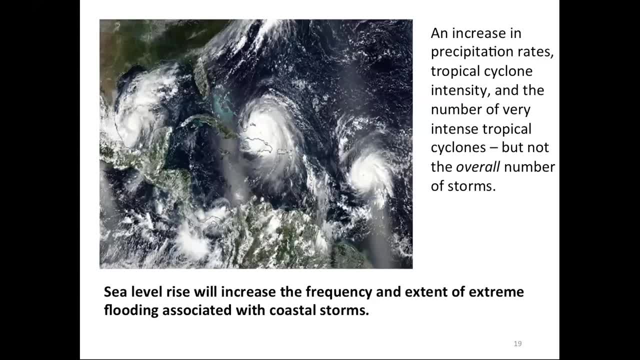 can't rule out the idea that there could be- could be fewer of those events And even though the balance of evidence suggests more of the strong, powerful hurricanes you know, probably can't rule out the idea that that could be wrong, given that upper ocean is only one of the key drivers. right, We also got to be. 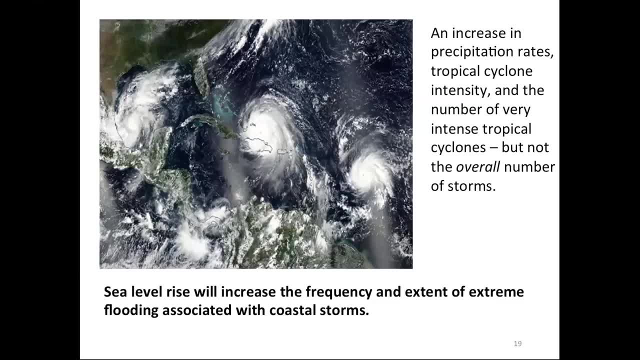 thinking about things like aerosols in the air, dust in the air, temperature of the upper atmosphere, amount of moisture in the atmosphere. what's going to happen to the sort of initial pulses, these low pressure systems coming off the African coast, for example, that are key to our sort of Atlantic? 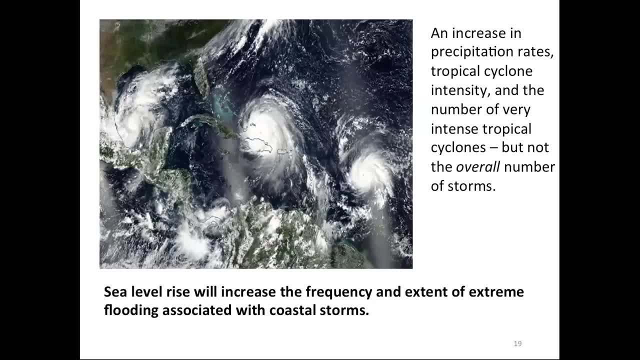 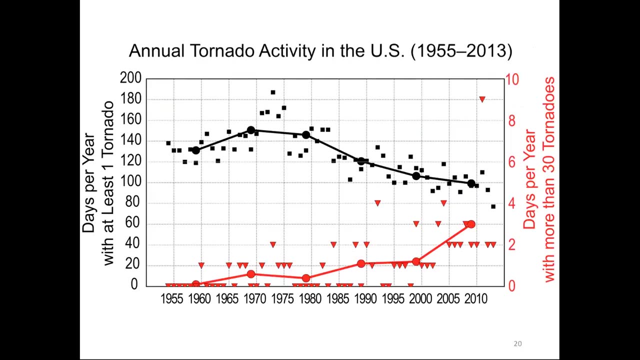 hurricanes. So this is a good example of a place where there's, you know, you know- more nuance, even as, from a risk management perspective, it probably makes sense, almost certainly makes sense, to think that the strong hurricanes will become, become more common Tornadoes, way outside my area of expertise. it's a 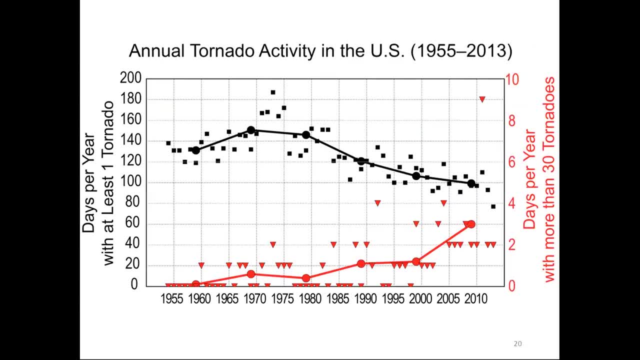 given that a lot of you on this call could could tell me much more about this than I can, So I'm going to go ahead and get started. That's probably true for a lot of the things I've talked about. Certainly it's true for for tornadoes. I tried to keep up a little bit with this literature. I 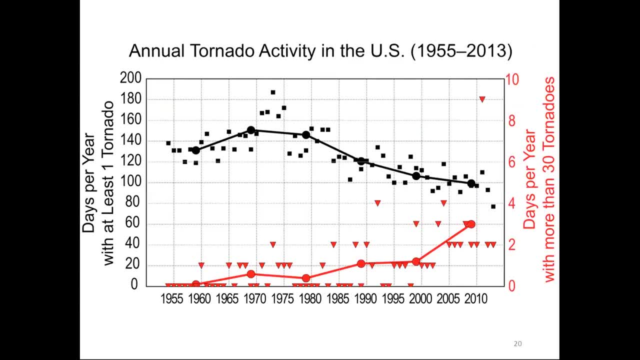 would you know, sort of tend to argue that you know. the first order statement would probably be: if we look at the historical trends, you know no clear and compelling evidence, probably, that the days per year with at least one tornado is changing in a meaningful way with climate change, Although you know some. 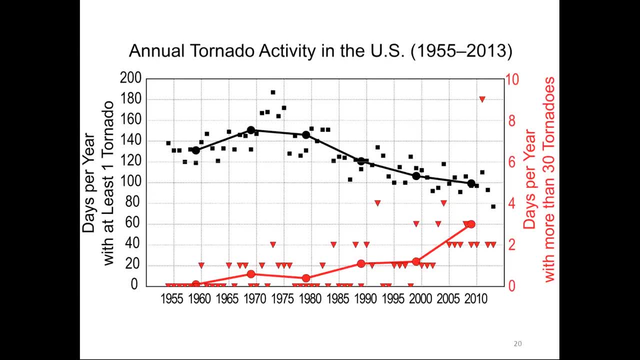 evidence. you know- I'm sure we could talk about data sources- how easy it is to track tornadoes and how that's changed could be responsible for some of this upward trend we're seeing in days per year with more than 30. These sort 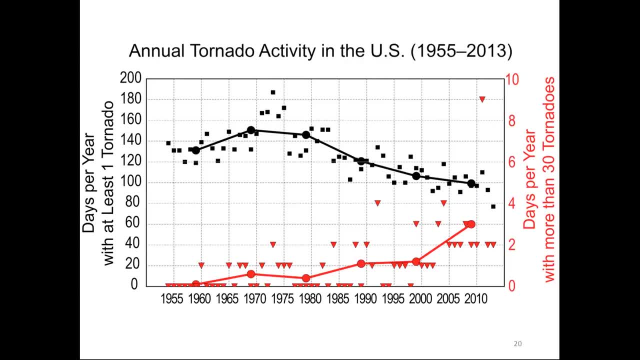 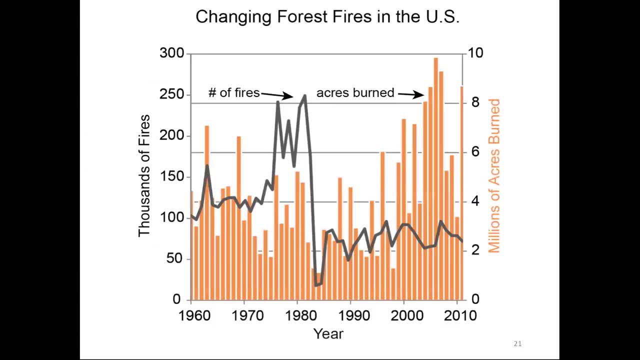 of cluster events again is way outside my area of expertise, but I wanted to put it up there because I'm sure it'll be of interest to many of you. How about wildfires? Here you know, we can you know again. look at multiple metrics, The. 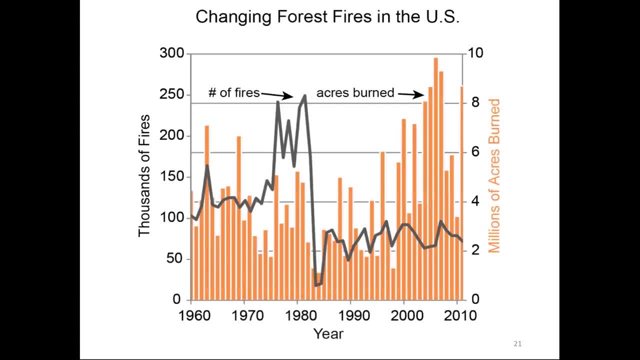 number of fires you know where. you know be hard to make sure they're not, as any case, that there's been an upward trend, but there is, you know, strong evidence that we're seeing more of these really big fires burning more and more acres. I think this is another. 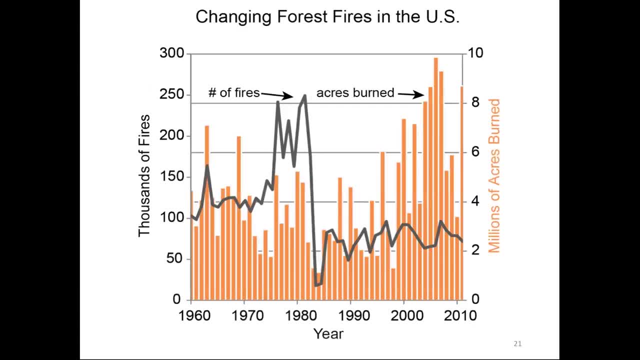 good example of unpacking. how much of this is climate change, how much of it is higher temperatures leading to moisture deficits, plants drying out, trees drying out, You know. certainly higher temperatures make it much easier for that to happen. That's part of the story. It's probably 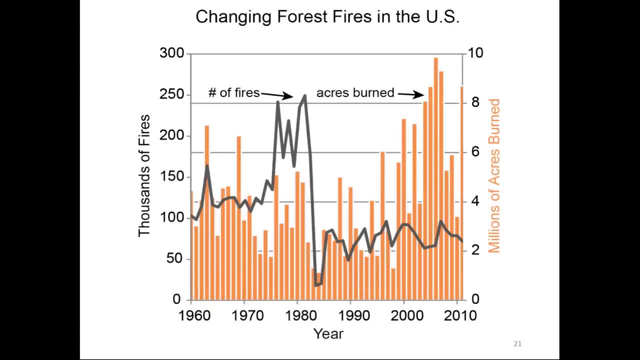 easier to settle that piece than the interannual precipitation. you know where natural variability still tends to dominate in most of these places. relative to a climate change signal, There may also be a component here to what's referred to as WUI right: People moving into the 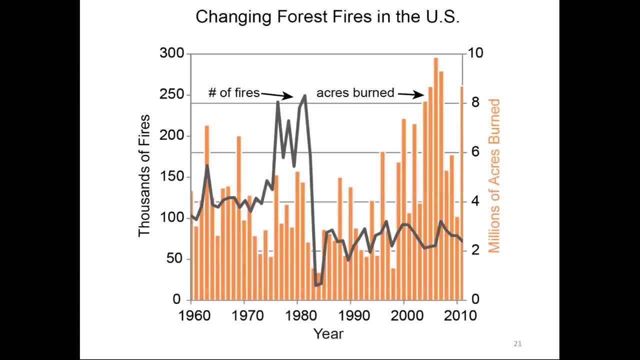 wildfire urban interface potentially starting more fires. That may be part of the story as well, as well as, more generally, changes in land use. You know forest management practices part of this story as well, But it's reasonable to say from a physical sense. you know, we know temperatures have been going up and we know 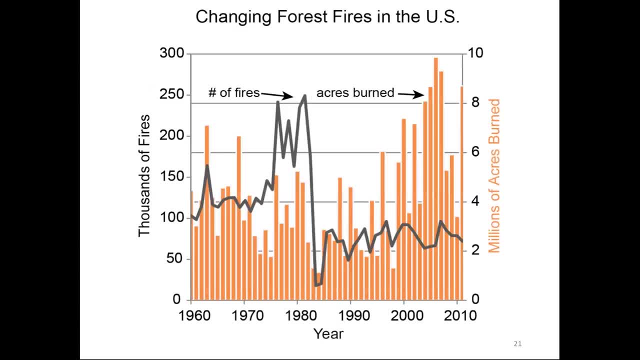 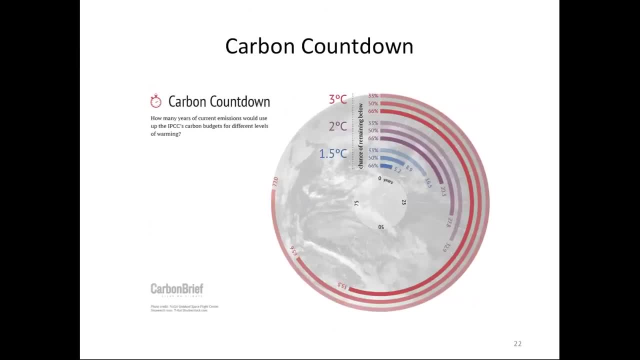 that, all things being equal, that can give you a lot more fire damage. That's part of the story. just how much I think is difficult to unpack. Okay, I'm almost done. I have a few more slides I want to show. You know, I've intentionally focused on historical trends, you know. but now 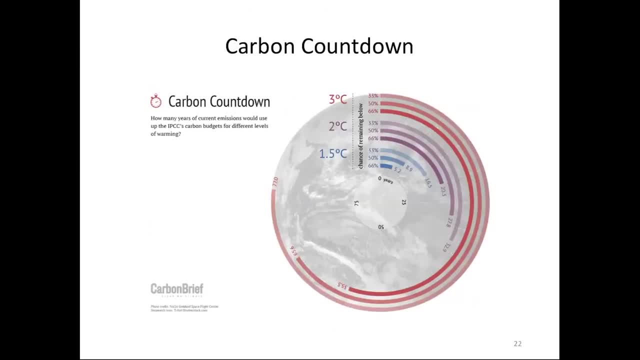 I want to spend a little time sort of thinking about where we go from here. So a little context. we've had about a 40% increase in the amount of carbon dioxide in the atmosphere directly due to human activity, land use changes and especially the burning of fossil fuels. 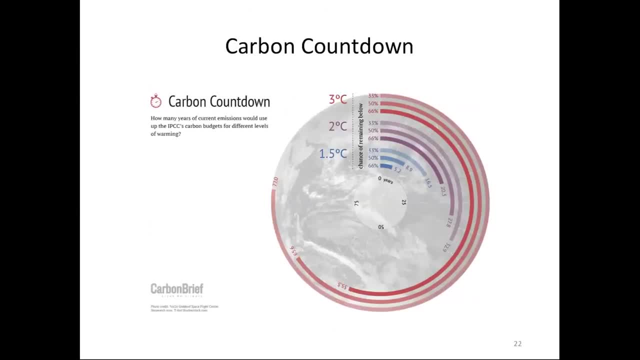 Had about one degree, a little less than one degree Celsius of warming globally during that time. If we want to avoid seeing that some of these extreme event trends accelerating, we need to dramatically reduce our emissions Further. we push carbon dioxide concentrations away from where they were pre-industrially. 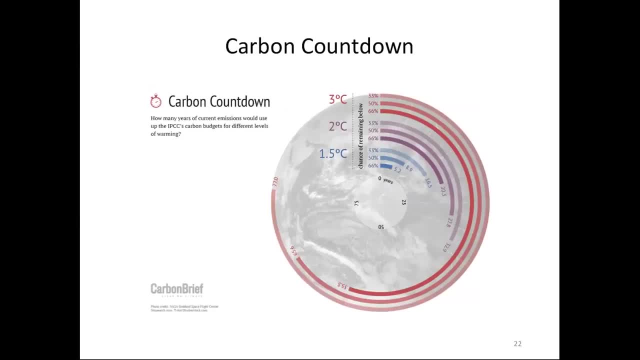 They had been about 280 parts per million. Now they're over 400.. Even if we reduce our emissions a little bit, as long as those concentrations keep going up, we're further from the equilibrium of 280, which means an acceleration of the types of changes. 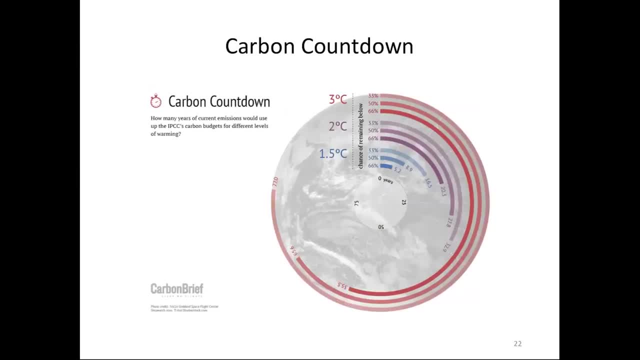 that we've been talking about. To actually turn that around, we need to reduce emissions to such a dramatic extent that the concentrations actually start to fall. So this is a major challenge requiring huge changes in everything from our energy usage to, you know, any number of aspects of our lifestyles. If we want to have a good chance of 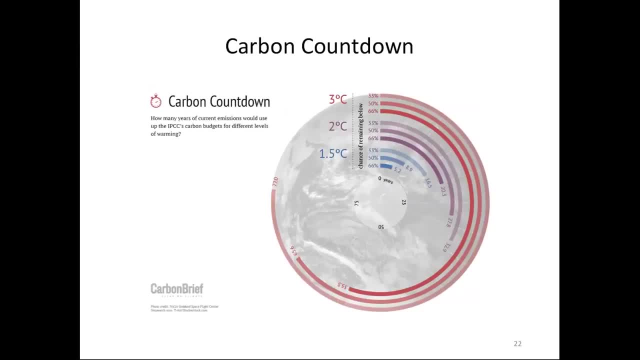 limiting ourselves to just two degrees Celsius of warming, keeping in mind that you know, carbon stays in the atmosphere a long time, so we're already locked into some more warming, No matter what we do to have even just a 50-50 chance of not blowing through two degrees of. 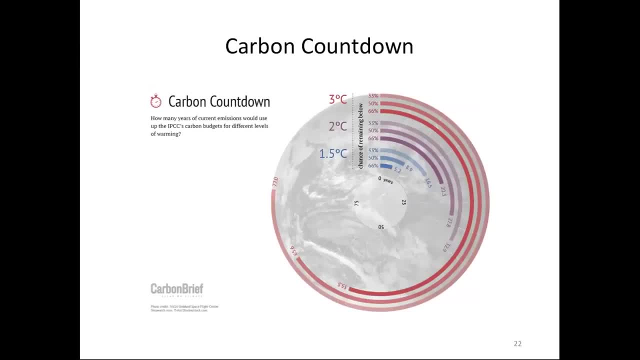 total warming and again, we've already had almost one degree. we really have only about now less than 25 years. This figure is a few years old, not the 27.8 that you see there in medium color purple. We have less than 25 years where we could emit globally greenhouse gases. 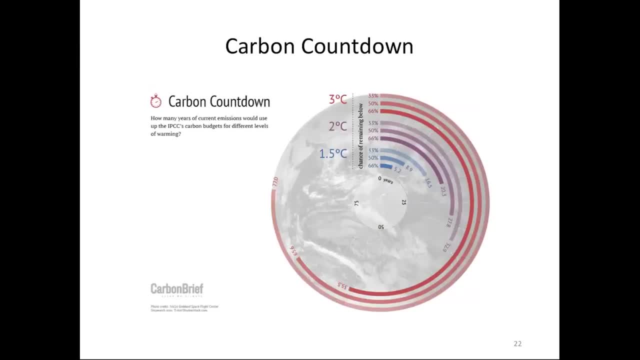 at the level we've been emitting them in recent years. At that point we'd have to immediately go to zero the next year, which of course you know, given our reliance, given that we don't have substitutes currently for things like aviation fuel, is just one example, you know. 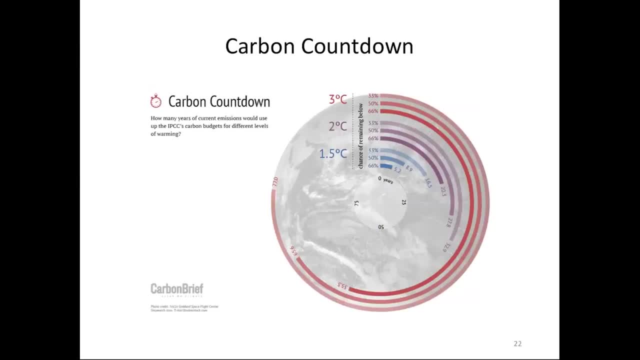 you see the scope of the challenge and the urgent need to dramatically reduce emissions, Or what right? Let's talk a little bit about the future here and I'll just tell you about sort of end with some of the things that I've been thinking about these days. 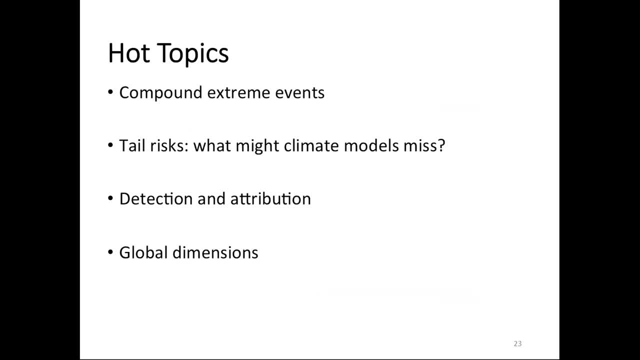 So first some hot topics I didn't really have a chance to to get into. A lot of people talking these days. I'm sure you are too many of you about compound extreme events. Can't just think about one variable. how are they interacting? Is there? 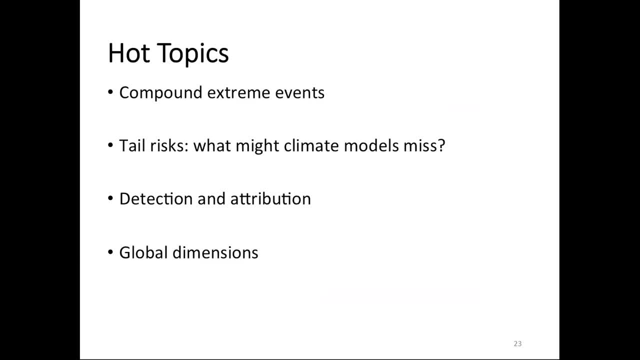 correlation in space between some extremes. If multiple bread baskets around the world get extreme heat and drought during the growing season, what that might that mean for global food security? If Boston gets sequences of nor'easters one after the other more often in the future, how does that modify vulnerability and risk relative to thinking about events? 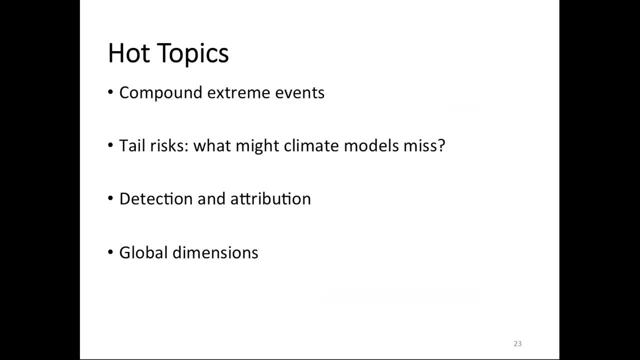 individually? Or what if you have a heat wave right after a tropical storm knocks power out? Compound extremes critical to risk assessment. I've talked a little bit about tail risks. What might climate models miss at either end of the spectrum? Critically important if we're thinking. 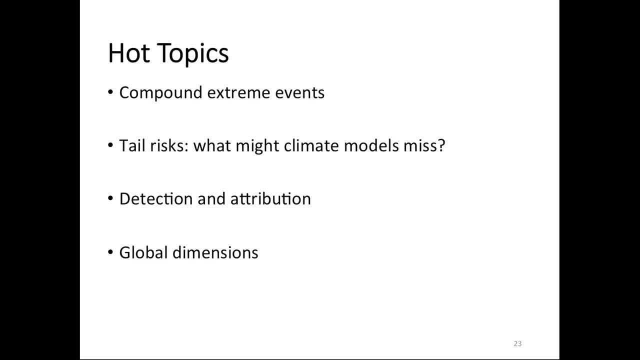 about things like nuclear reactors, nuclear plants that may be near sea level. You know, critical infrastructure of high value. as a couple examples, A lot of people talking about detection and attribution of extreme events. now, As we can attribute the frequency of some of these, 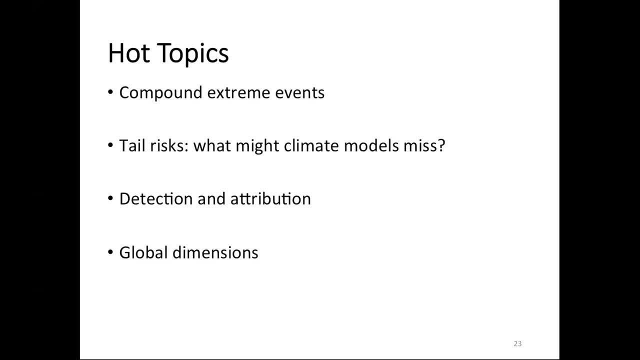 events or a portion of what happens in the events- portion of the rainfall, for example- to this increase in greenhouse gases. that potentially opens up some interesting doors in terms of risk communication, Some people even beginning to argue that sort of liability conversations about sort of responsibility for fossil fuel emissions. to date, 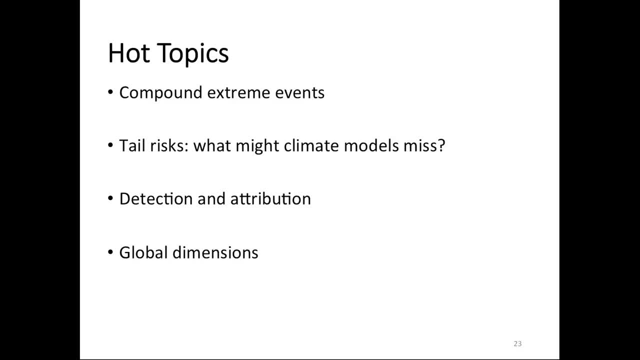 could be brought up more and more in the context of human contributions to damages associated with extreme events such as Sandy, to name just one. And what are the global dimensions of extremes? We've talked a lot about the US, but how are we all affected, you know, by changes in other? 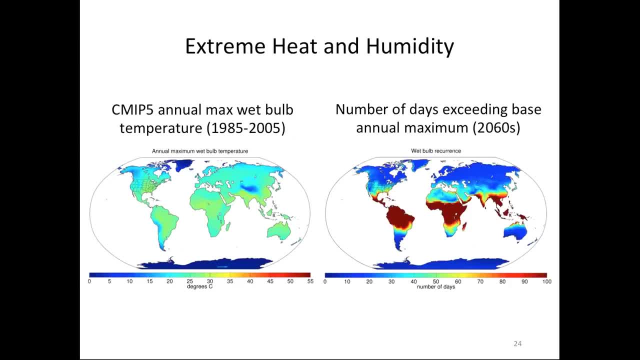 places too, in extreme events. An example of a compound wet bulb: this, this combination of heat plus humidity, Showing on the left here. this is climate model results, for you know where you expect to see the highest wet bulbs. you know the highest wet bulb day, that link of high. 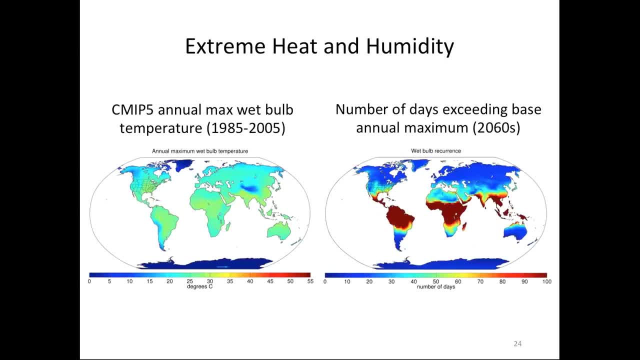 temperature and humidity in the historical period shown on the left. So you see the higher values sort of trending towards yellow in some parts of the tropics, but not exclusively the tropics. You can see some fairly high values over parts of the eastern US. 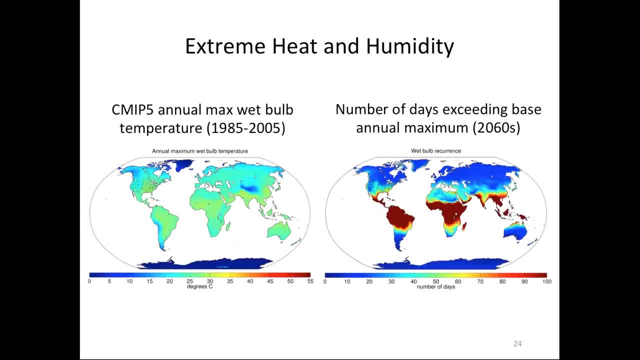 And then you can go to the right and say: for whatever that wet bulb temperature, that combination of temperature and humidity that used to happen once per that historically happened once per year. say, it's a wet bulb of 30, you know, as we go to the future mid-century, this is a scenario where 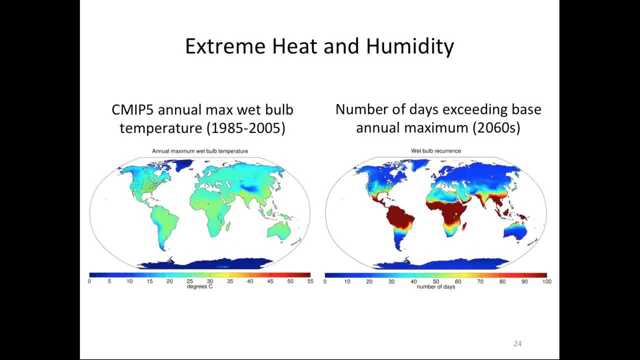 we emit a lot of greenhouse gases. how many days per year is that particular threshold of temperature and humidity, that high threshold, going to be crossed in the future? You can see again how many times we emit greenhouse gases. if we continue to emit a lot of greenhouse gases. 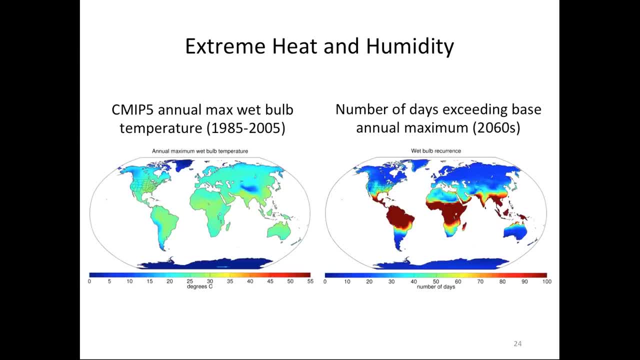 only that frequency changes just within a generation or two. If we continue to emit a lot of greenhouse gases- for parts of the US essentially two months per year, 60 days or more- you know where you're having that extreme threshold that historically has only happened once per year. Again, as with all, 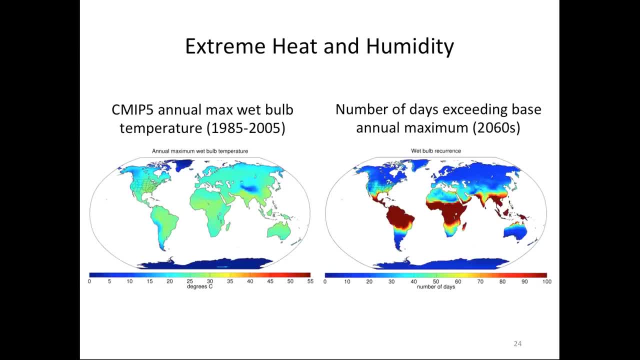 this don't focus on these precise numbers. These are climate model outputs. Different things are going to be happening to some extent at local spatial scales. point here is that we're talking about more than an order of magnitude change associated with just a relatively small amount of warming. So this is, I think, a risk that's been understated And to 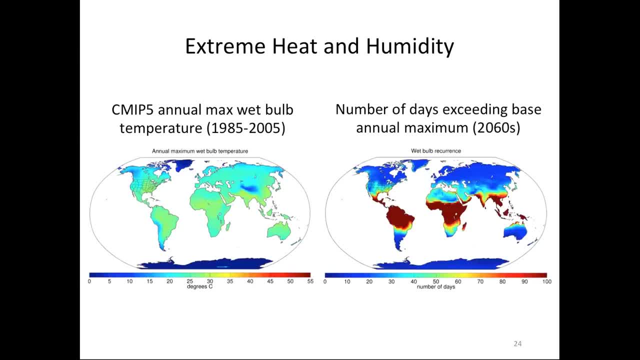 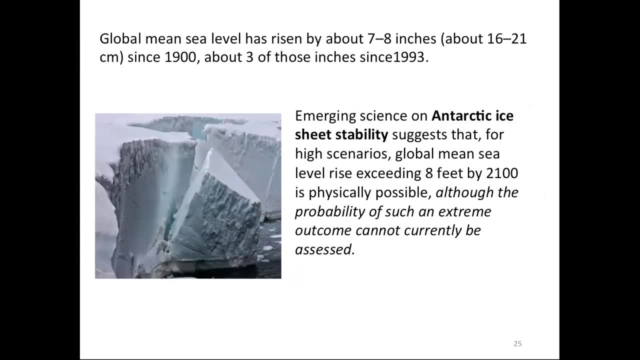 really understand it. we need to think about temperature and humidity and how they interact together. It has such a big impact on our ability to cool ourselves. Okay, Tail risks Things that climate models may not capture well. The iconic example certainly is sea level rise. 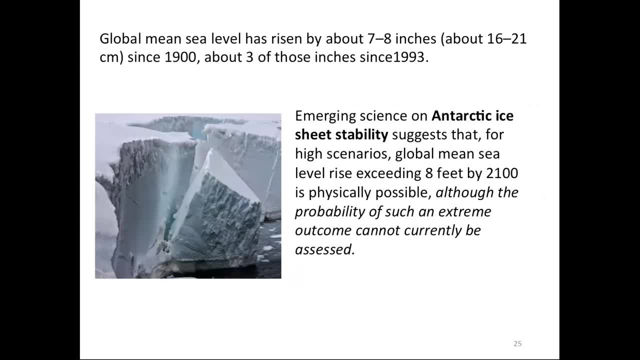 You know, we've understood now that some of the many ways that an ice sheet can melt that ice that sits on land, a lot of it happens at really fine scales that climate models aren't able to capture that well And we're becoming more and more concerned as those greenhouse gas concentrations. 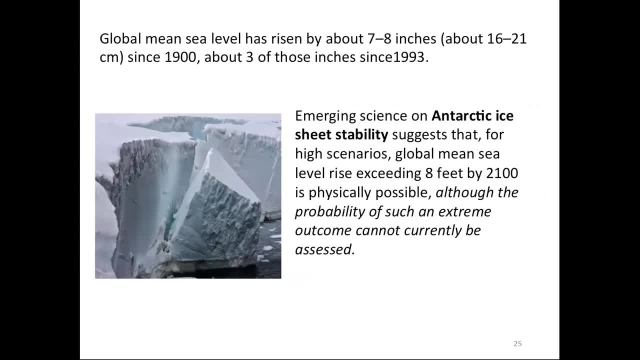 go higher and higher, that we may be unleashing, you know, fundamental changes, accelerating processes that, even if we were to lower greenhouse gas concentrations, might prove hard, And so you know we don't know where those tipping points sit. hence the urgent need to, you know, reduce our 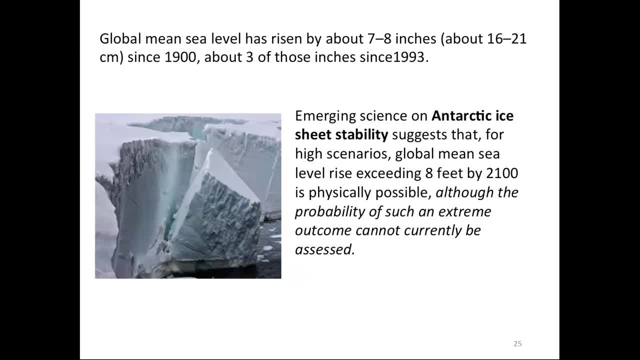 emissions, So we don't go further outside of that envelope of what we've experienced, you know, and so that we don't sort of open the door to these sort of Frankenstein solutions such as sea level rise, you know, far in. 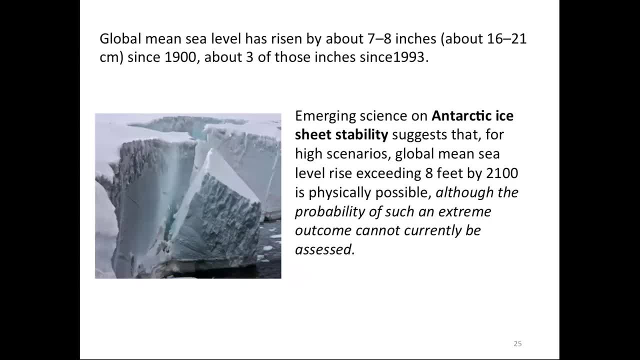 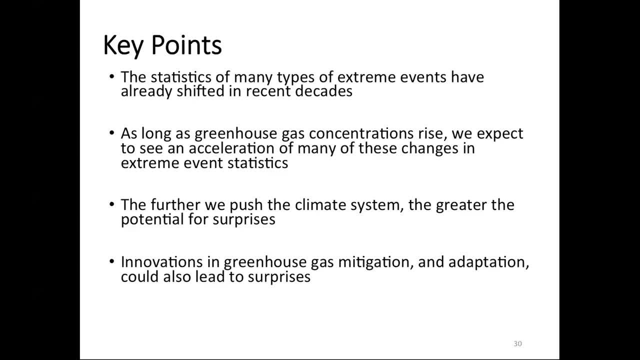 All of our sort of assumptions about how things work, that guide everything we do, that guide our meteorology, as one example, may not hold up to the same extent in the future. So this, of course, is the basis of this argument for why we need to reduce our emission so dramatically and why adaptation and resilience are so critical. 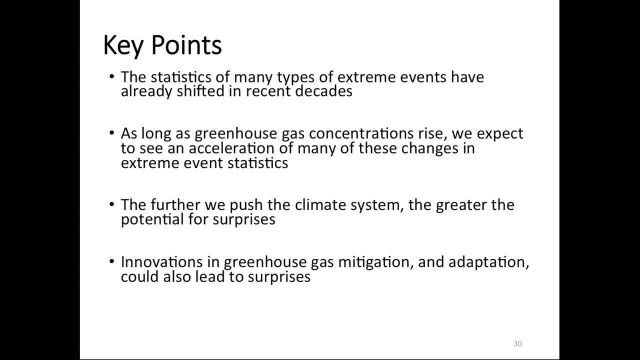 Maybe we can get tipping points and surprises on that side to really help us out. We've seen how quickly the cost of renewal collapses. We've seen how quickly the cost of renewal collapses. renewables, solar and wind generation are dropping. We see advances in battery storage technology. 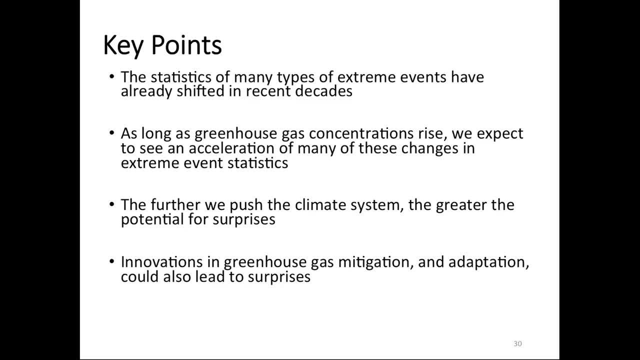 electrics. You know we're not that far away potentially from some tipping points in terms of the economics working in the favor of renewables And, on the adaptation side, maybe some surprises too, You know, just to give one example, hearing more and more about 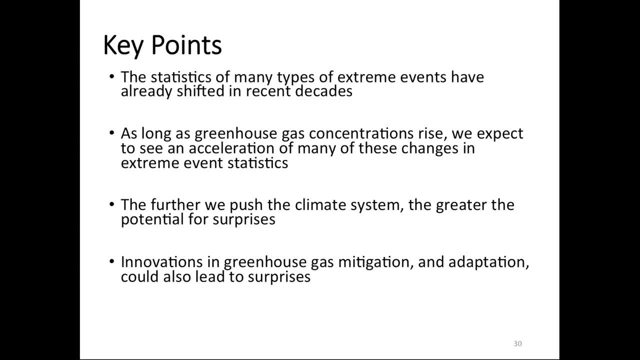 companies like Moody's, you know, that are sort of critical to underwriting bonds for municipalities and other groups, demanding really that you know climate hazards of the type we're describing here today be considered in the planning as people look to the future. 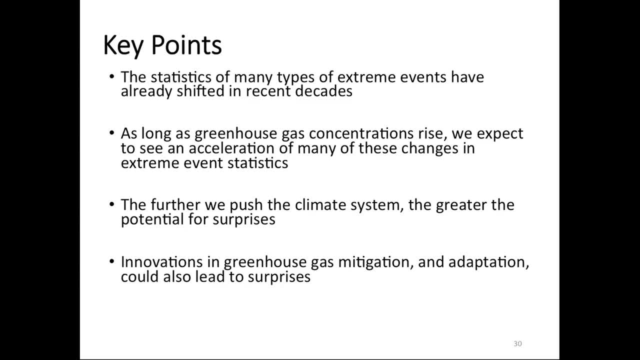 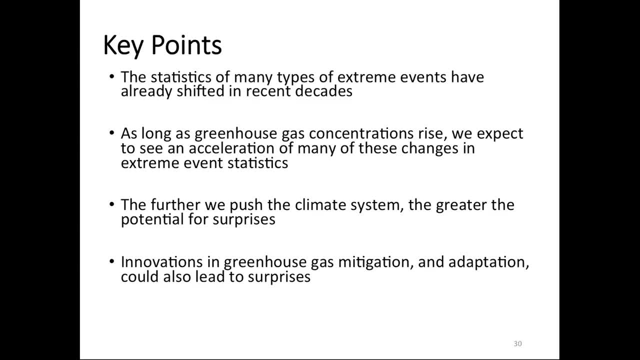 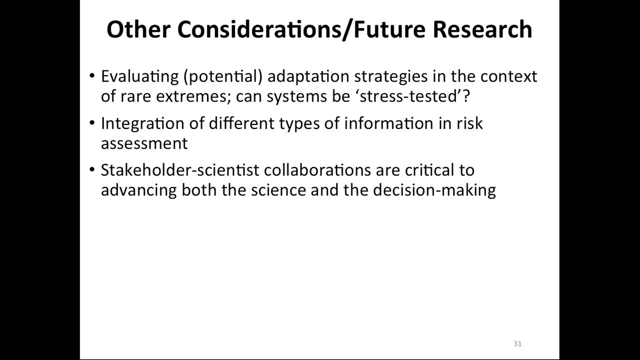 And I think that's going to be a big problem. And I think that's going to be a big problem. How can we evaluate some of these adaptation strategies underway- green infrastructure, storm surge barriers- in the context of rare extremes? Can we stress test some of these adaptations before the next Sandy or Harvey happens? How do? 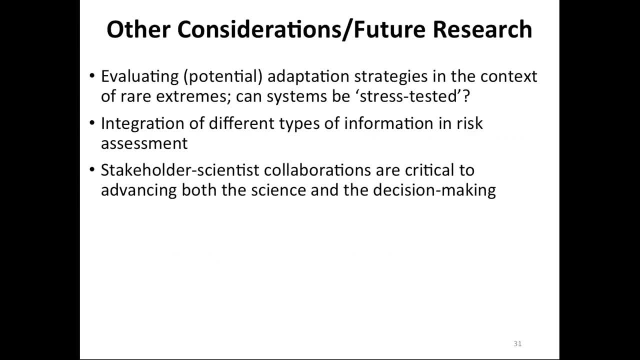 you evaluate some of these adaptation strategies before the next Sandy or Harvey happens to do that. Is that a role for scientists? Is that engineers? Is it all aspects of society? How do we do risk assessment? that's not just climate models, that looks at the historical. 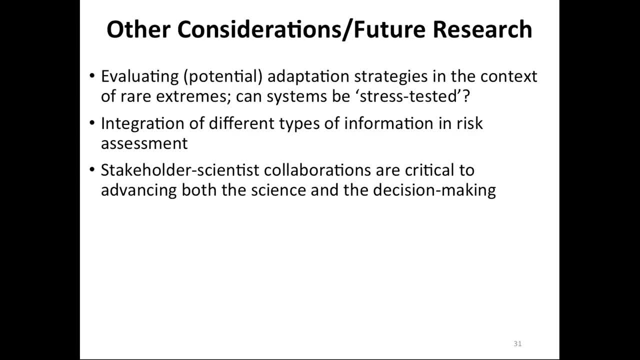 data that looks at physical processes, that looks at expert judgment. That's how we can do our long-term planning and stakeholder scientists, collaborations, collaborations with you all, across all of society, I think, are going to be key to those kind of processes. So I'll end there. 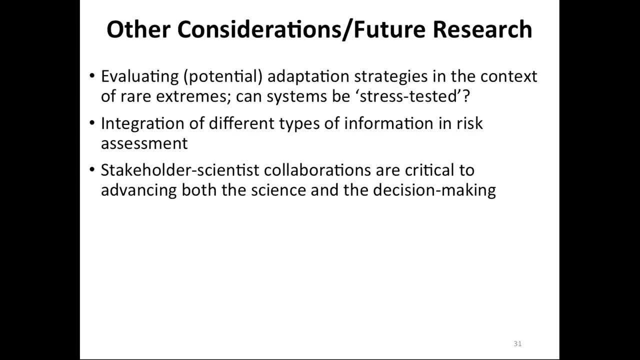 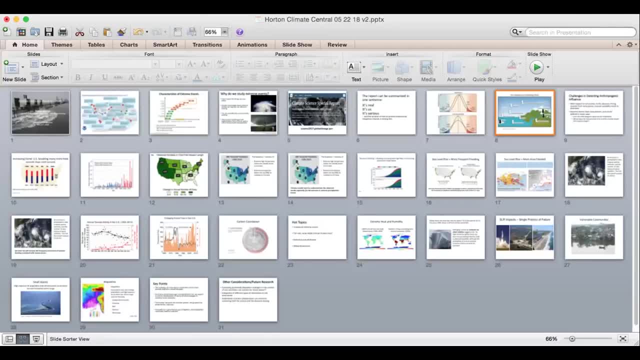 Thank you, Riley. thank you very much. I appreciate all that good information. It is a lot to take in. no question, I'm going to leave control of the presentation with you for a minute as we attack a couple of questions here real briefly, if there's something else you want. 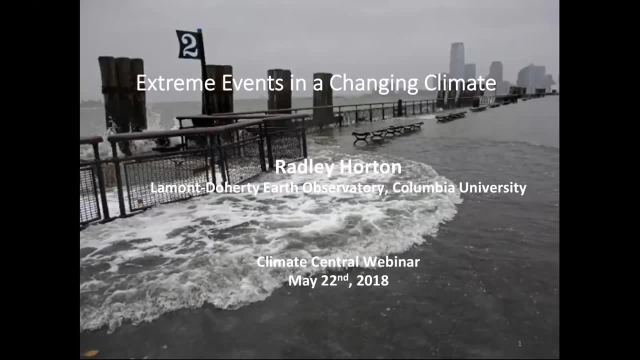 to pop up while we do this. One of the questions I had, real briefly, was: is there any good way- this is not an easy question at all, but how to unpack some of those things you talked about earlier in terms of society versus meteorological impacts vis-a-vis flooding. 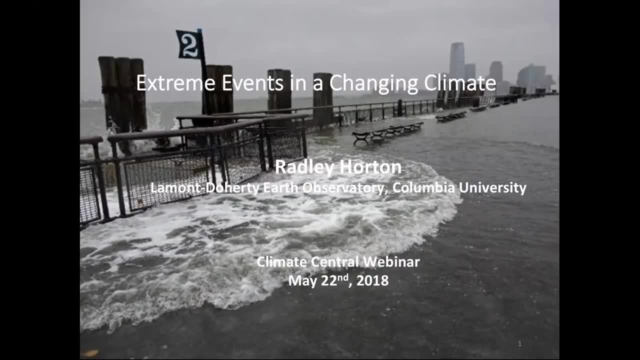 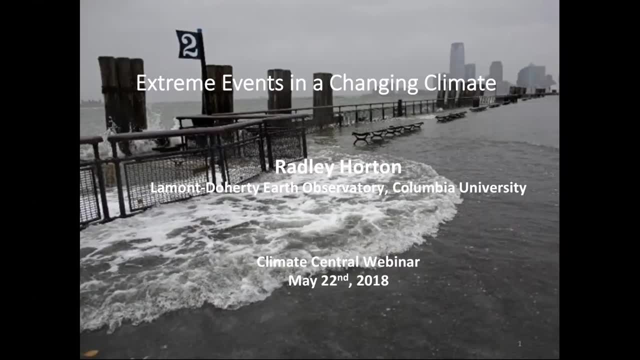 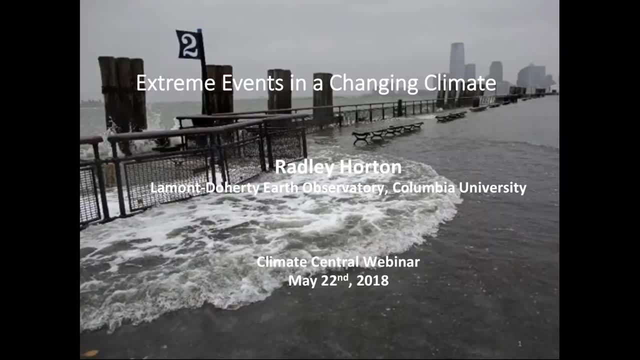 in the Gulf area, for example. Of course, in the real world we don't have that rich station-by-station detail going back 100 years, certainly not hourly, So we're never going to know exactly. you know before climate change, precisely what was the one in 100 year hourly rain event. one in 100 year, you know, three day rain event. 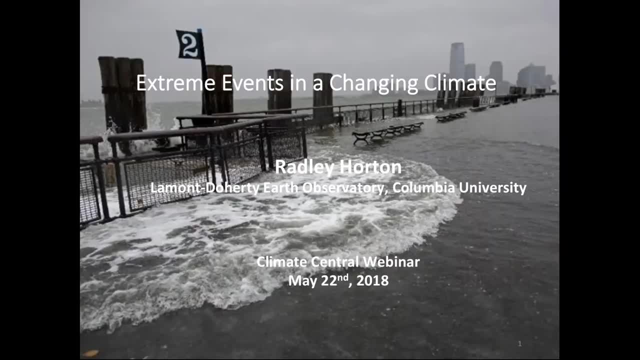 But you know, we do know there are things we can do. right, We can run models over a historical period with the greenhouse gas concentrations of what they were back then compare how much either rainfall you get in those simulations or something else that we associate, you know, with rainfall the amount of moisture in the air. 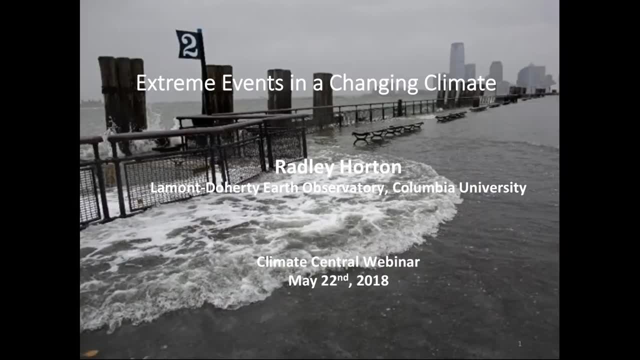 We can compare that to a climate model run for the present greenhouse gas concentrations. Does the model suggest that you should get more heavy rain event? That would be a good data point, I think. to get to your question, you know we need, you know, the input of hydrologists for sure. 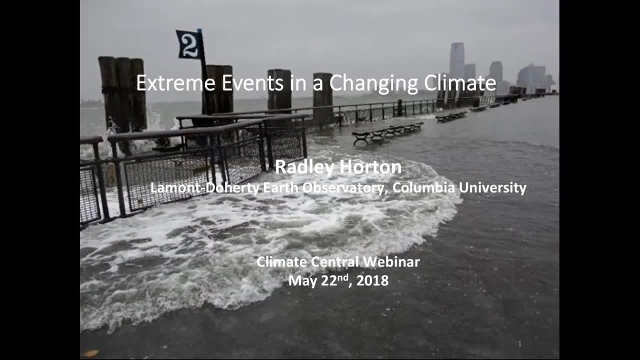 That would be one you know, obvious, obvious, dimension, Land use changes. you know engineering. I think that's, you know, a grand challenge And you know we're probably never going to get you know down to you know a few percent precision in terms of responsibility. 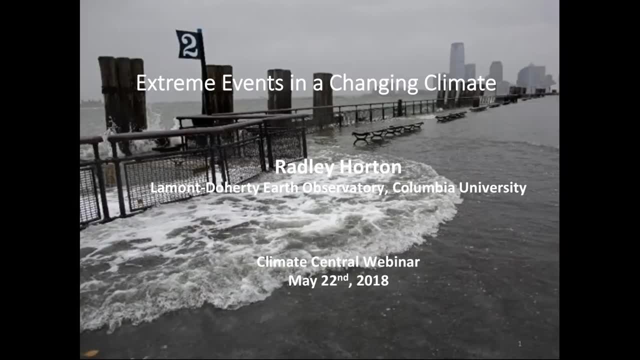 But you know, there's, you know, I think clearly there's, clearly there's a role in the climate. We can also learn things by leveraging other places right. We can. You know, to some extent we can treat the entire Gulf Coast, for example, as a region, a region that differs. 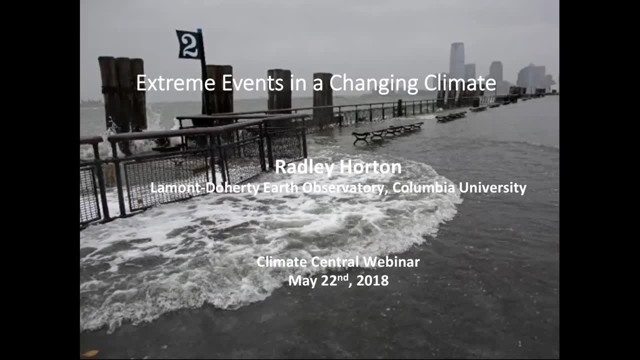 But you know there's some additional power we can gain from aggregating storms across larger areas. I'm sorry I don't have a better answer to your question. I think it's, you know, a really important and really challenging one that points to the need to engage all of society in these questions. 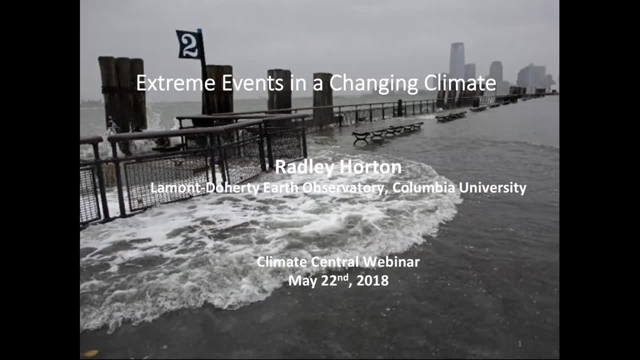 Yeah, I mean it is a difficult one to be sure. Yeah, we go back and you run these hindcast models in these different Scenarios to try to get some some idea. So it is certainly not an easy proverbial nut to crack. 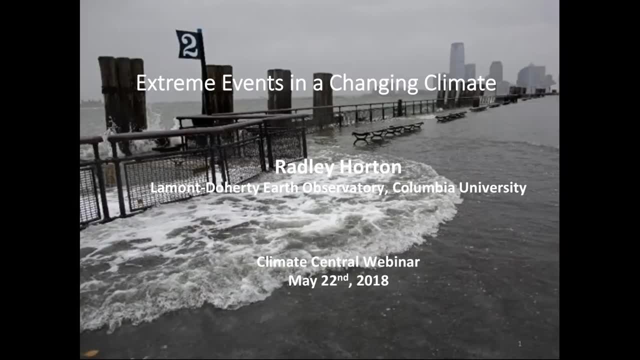 We did get one other question in regarding ice storms. of course, next to hurricanes and tropical systems, That's big, big damage to electrical utilities in a warming climate. Has there been anything looking at the increasing frequency of ice storms? This is another one that I don't know much about. 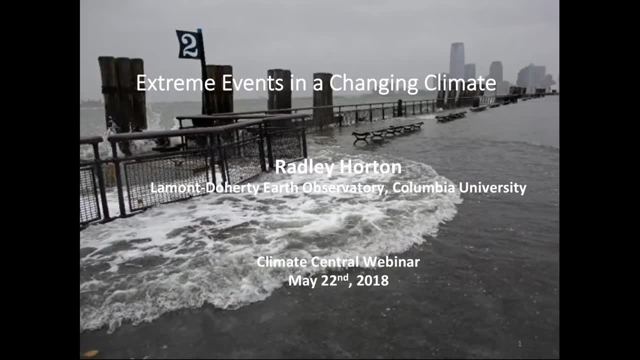 But I'll I'll try to summarize, you know, my- you know, sort of limited knowledge on this And maybe there's a way offline that others with with more expertise can can sort of fill in the discussion. You know, my overall understanding is that, you know, ice storms again fall in this category of rare events where the natural variability can be really large relative to any trend. 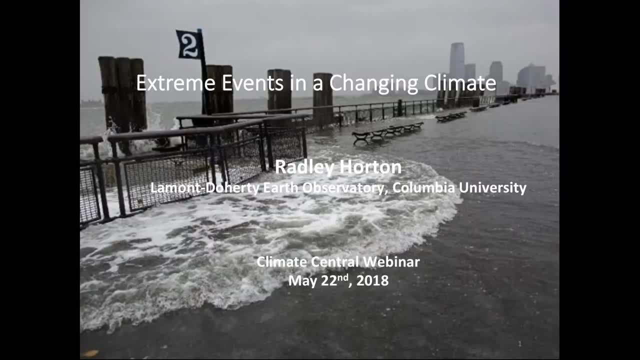 I haven't seen studies suggesting a strong anthropogenic human trend In ice storms. that's kind of the extent of my knowledge. I'll just point out though, from a process perspective, you know one might be tempted, you know, sort of initially to think: oh, you know, warming temperatures might give you less. you know instances when you could have ice. 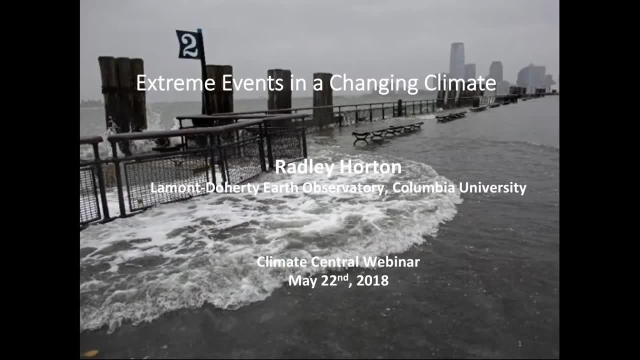 But of course that would be, you know, you know, way too simplistic, you know, just by having fewer freezes, But that's of course way too simplistic. Right, You know, we have to think about temperature profiles in the atmosphere, the amount of moisture in the atmosphere. 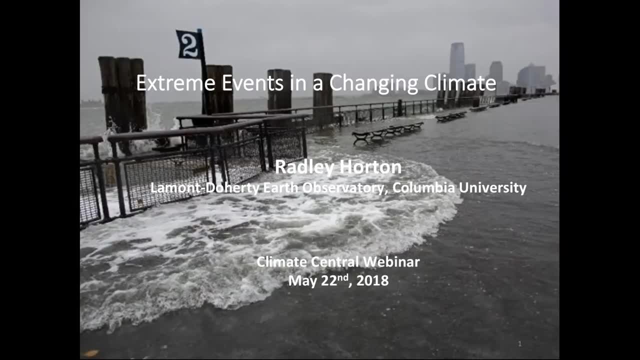 I don't think That sort of you know overall, you know an individual sort of explanation of the physics alone could, could could, answer this one, although those with more expertise could probably, you know, do a better job than I did. 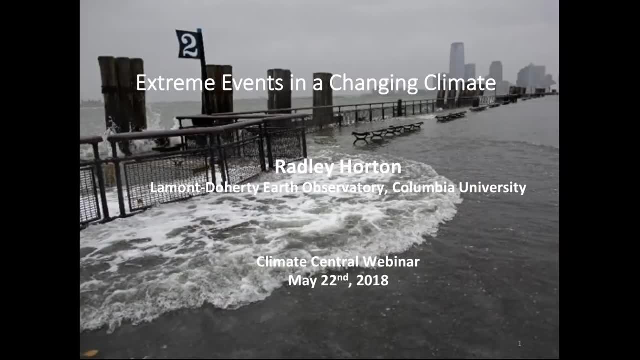 But I think you know this is one where the uncertainties are high And I, at least you know, haven't seen a study over the US as a whole that showed a long term trend one way or one way or the other in the context of this huge, you know, really big year to year variability. 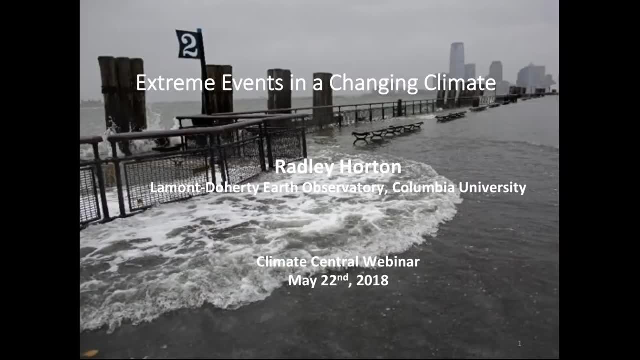 All right, Riley, Almost out of time. As I mentioned, Bernadette's here beside me, I know she had something she wanted to chime in as well. Bern, please go ahead. Bradley, thank you so much. This is fantastic. 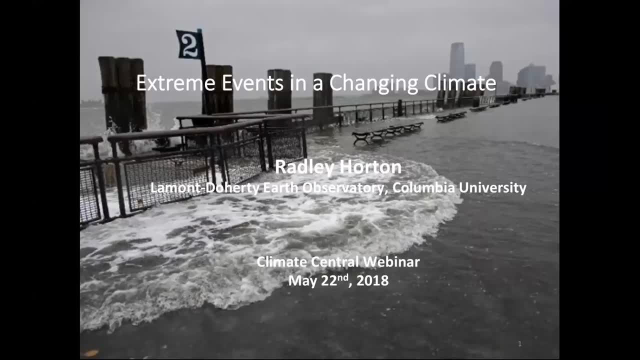 And I loved, in particular, your sort of foresight, bringing up the hard questions that we don't necessarily have answers to yet, but really are the areas of research that we need to focus on. And with that being the case, I'm kind of curious: just from your perspective, what's the most exciting area of research as it pertains to? 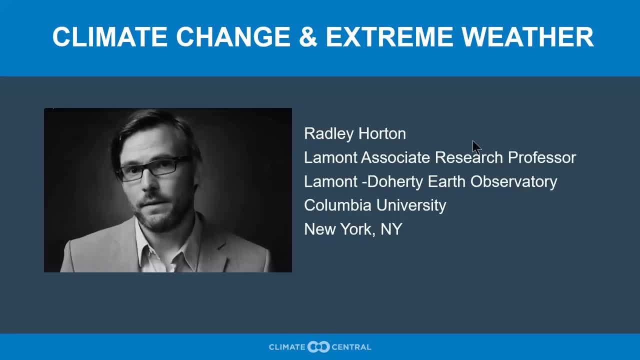 What's the most exciting area of research as it pertains to extreme weather right now that you're either a part of or that you are following? Yeah, that's a great question. I would say that I'm- you know, I'm very interested in this general topic of the compound extreme events. I would say 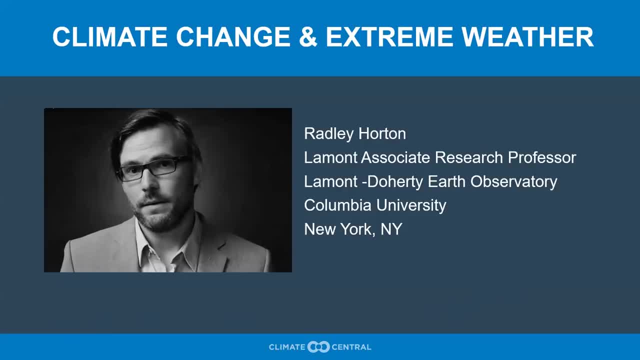 So, historically, maybe we looked place by place, event by event, and said: you know how might each place be affected by a particular heat wave? Now, taking this approach instead of you know, could we see a greater risk of simultaneous heat waves in multiple places or longer duration heat waves. 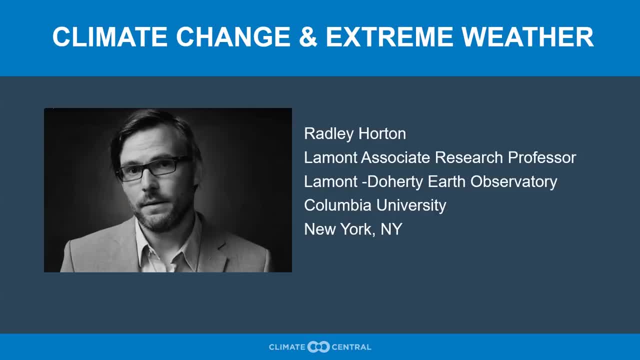 We think about the spatio-temporal characteristics of extremes and how those could change, for example, if the jet stream changes, You know, if we see less steering sort of west to east in the mid-latitudes in the future, A big if. but I think you know from a risk perspective something that's distinctly possible. 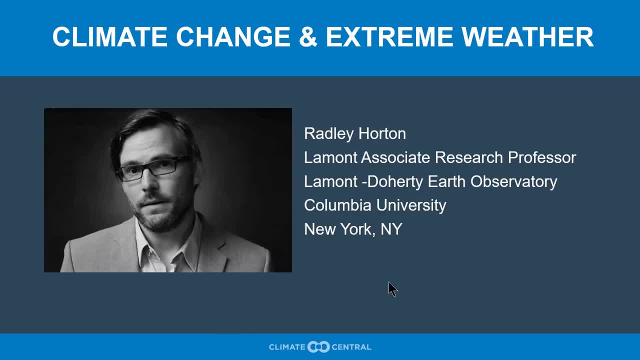 So what might that mean? It could point to some, you know, nonlinear surprises in terms of the ability of our food systems to respond, you know, as just one example. So speculative to some extent, but I think you know, critically important from a risk perspective. 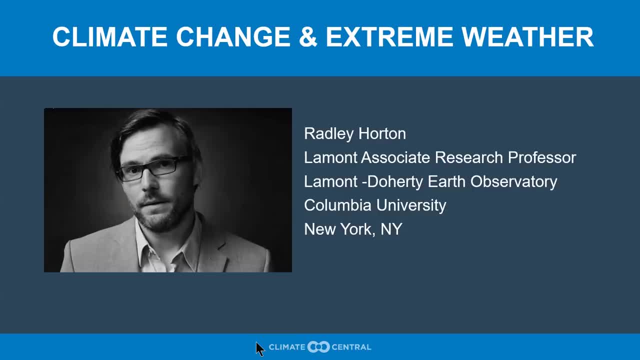 Thanks. That's really helpful And I know that that's a topic that's been brought up with the National Climate Assessments and in general too, In addition, how that reflects on our response system, And we saw that being stressed with the hurricane season. 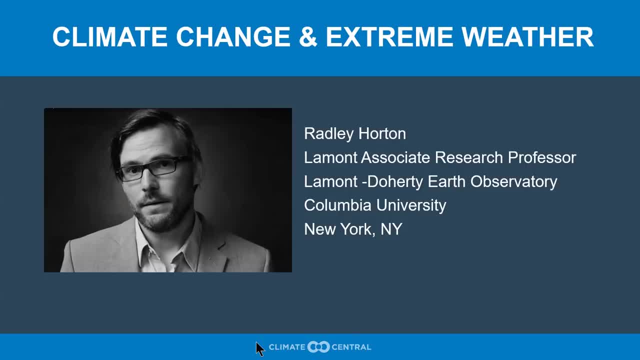 And then we just went through already and how these compound events could make that even worse. So thank you very much. I appreciate that. Thank you All right, Bradley. thanks again so much for spending time with us this afternoon. Appreciate you making the effort to spend some time with us today. 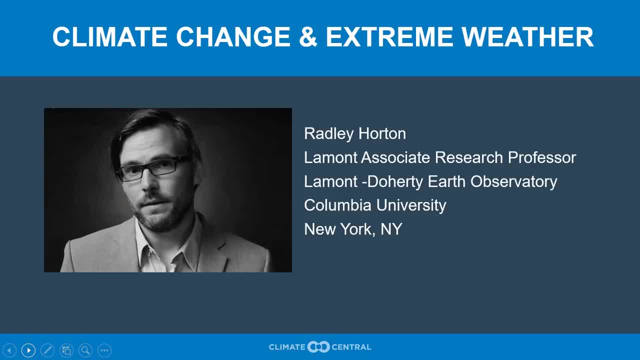 Thanks everybody You bet, You bet Absolutely. Also for those of you still on the line, be on the lookout for our next two Climate Matters releases Tomorrow. we examine droughts and deluges, Examine percent of normal precipitation. 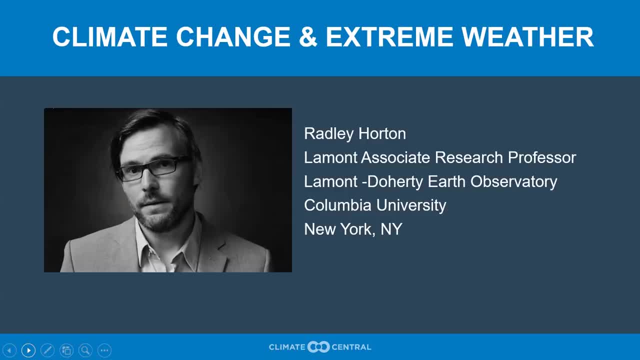 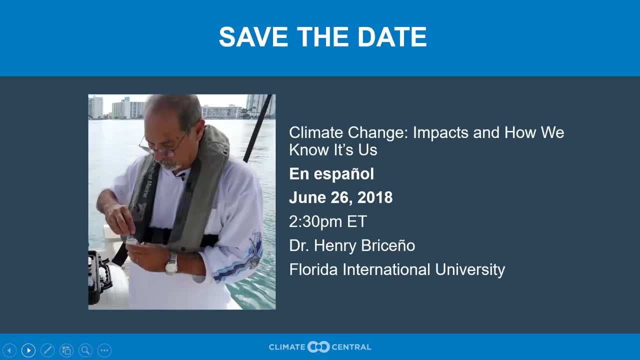 So far in 2018 for 244 cities across the country. And then the following week we'll have a new analysis on Atlantic hurricanes, just a couple of days before the next Atlantic hurricane season And right before we go, save the date.